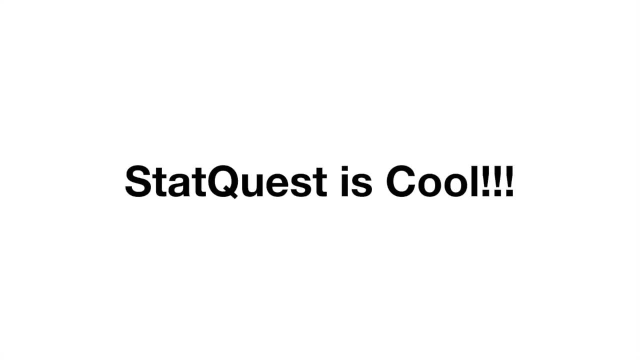 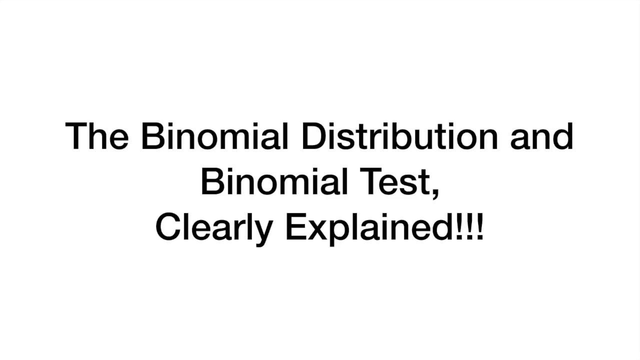 StatQuest is cool. That's my opinion. If you don't think so, then your opinion is inversely correlated with mine. StatQuest. Hello and welcome to StatQuest. Today, we're going to talk about the binomial distribution and the binomial test, and they're going to be clearly. 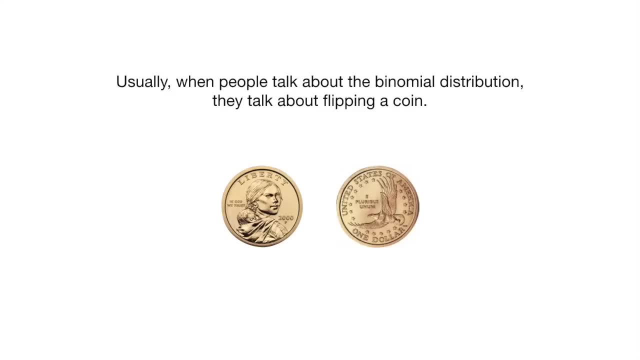 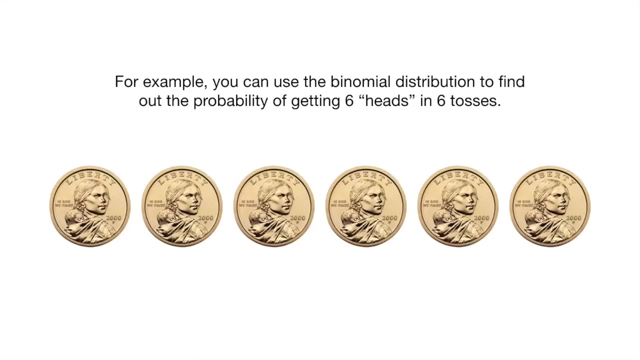 explained. Usually, when people talk about the binomial distribution, they talk about flipping a coin. A coin usually has heads and at least one tail. For example, you can use the binomial distribution to find out the probability of getting six heads in six tosses. But who really? 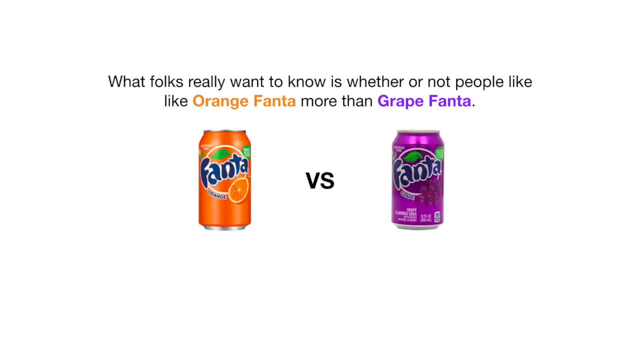 cares about flipping coins. What folks really want to know is whether or not people like orange Fanta more than grape Fanta. Which flavor reigns supreme, Or are they both equally loved? To answer this question, we can ask a bunch of people which flavor they prefer. 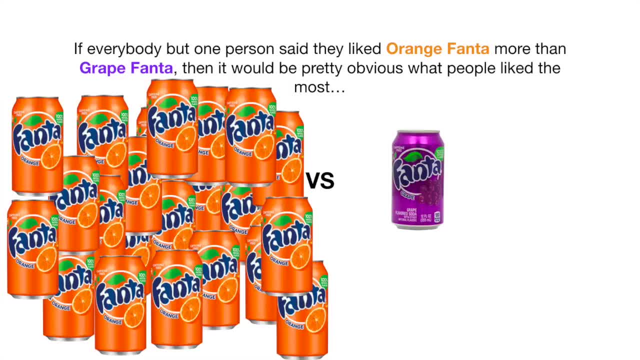 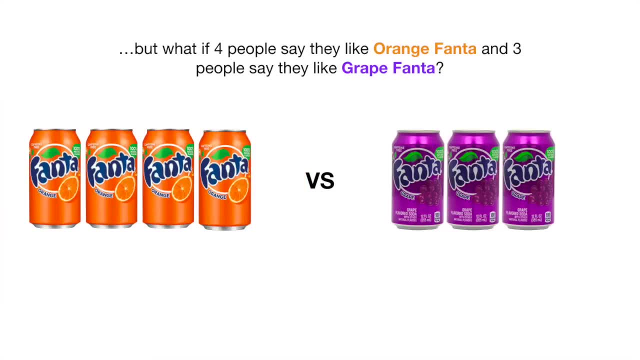 If everybody but one person said they liked orange Fanta more than grape Fanta, then it would be pretty obvious what people liked most. But what if four people say they like orange Fanta and three people say they like grape Fanta? Is that enough to be confident that most people like orange Fanta, Or could it be that people 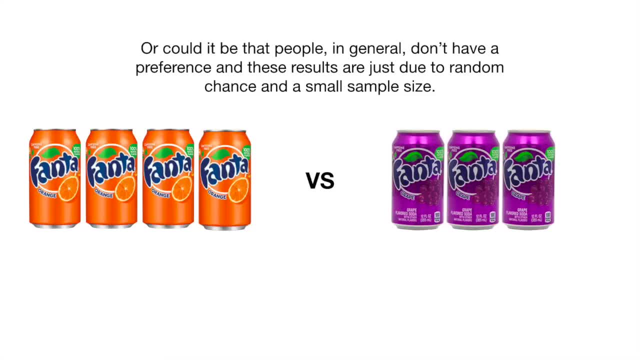 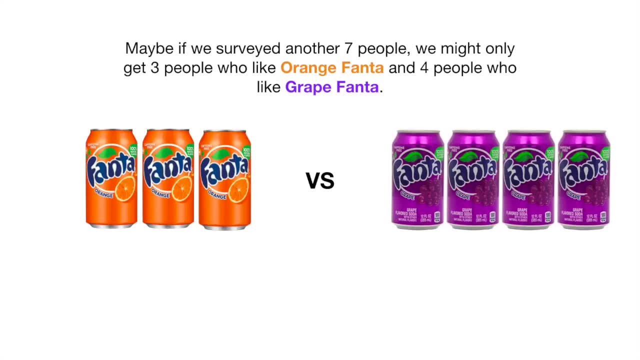 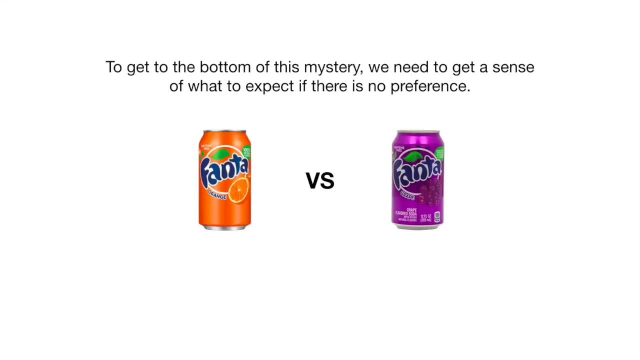 in general don't have a preference, and these results are just due to random chance and a small sample size. Maybe if we surveyed another seven people, we might only get three people who like orange Fanta and four people who like grape Fanta. To get to the bottom of this mystery. 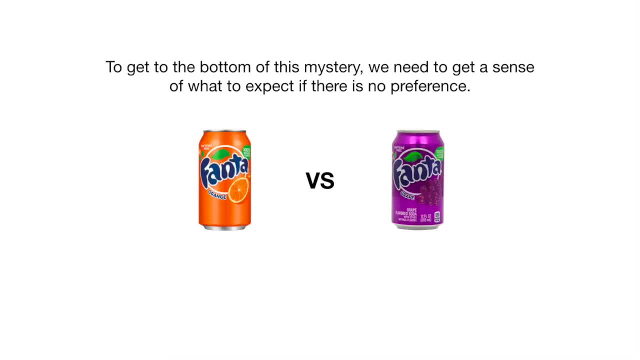 we need to get a sense of what to expect. if there is no preference, Then we determine if our survey results fit those expectations. If not, we can reject the idea that both Fantas are loved equally. The binomial distribution will tell us what to expect if. 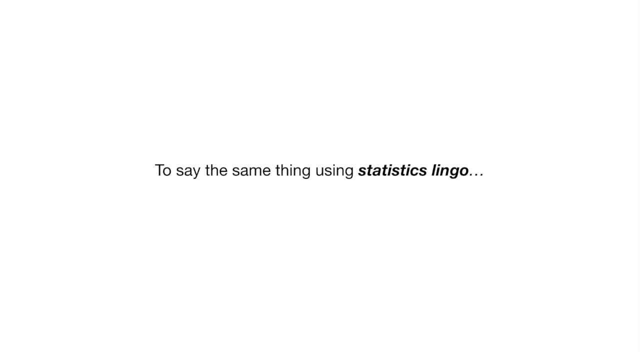 there is no preference To say the same thing, using statistics lingo, we will use the binomial distribution, aka the binomial distribution, to determine what to expect. if there is no preference, We plot the symbol c a, this nasty looking thing, to model what to expect. 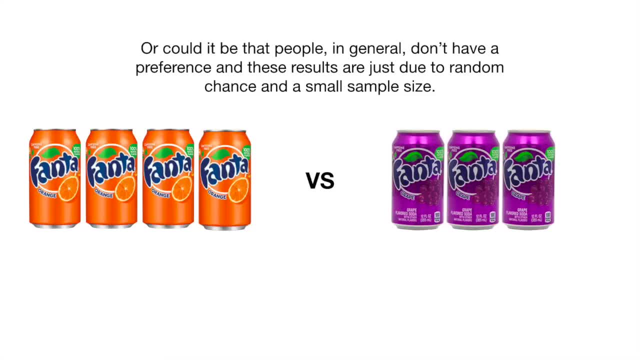 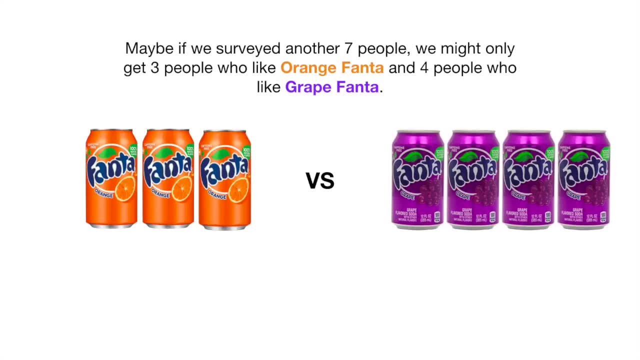 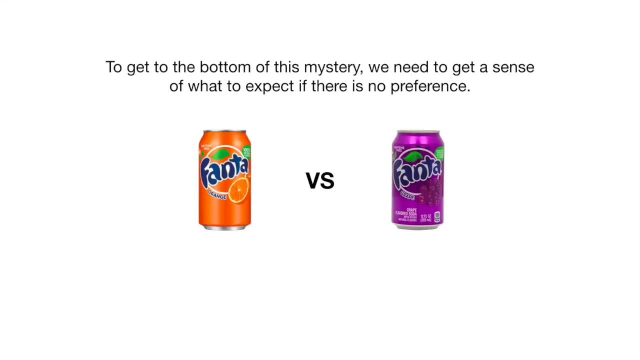 in general don't have a preference, and these results are just due to random chance and a small sample size. Maybe if we surveyed another seven people, we might only get three people who like orange Fanta and four people who like grape Fanta. To get to the bottom of this mystery. 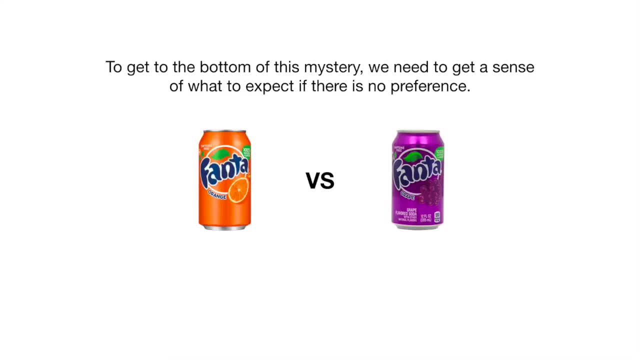 we need to get a sense of what to expect. if there is no preference, Then we determine if our survey results fit those expectations. If not, we can reject the idea that both Fantas are loved equally. The binomial distribution will tell us what to expect if. 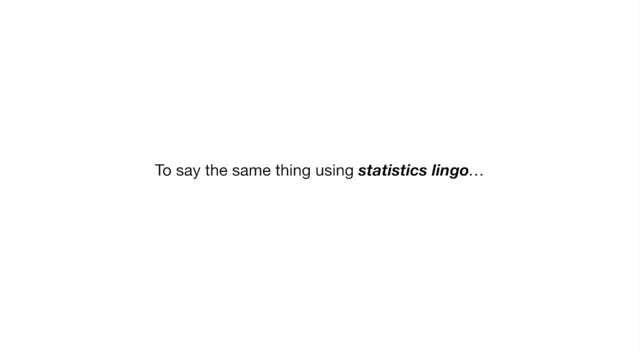 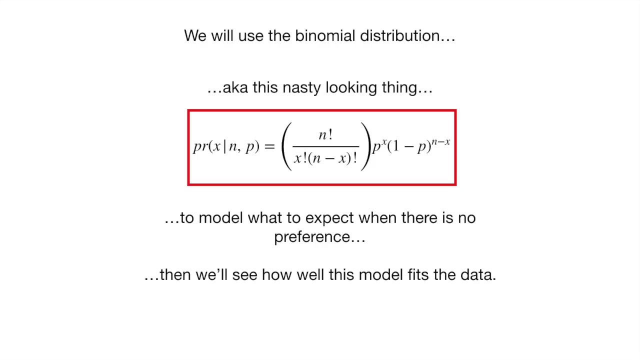 there is no preference To say the same thing. using statistics lingo, we will use the binomial distribution A, this nasty looking thing, to model what to expect when there is no preference. Then we'll see how well this model fits the data. 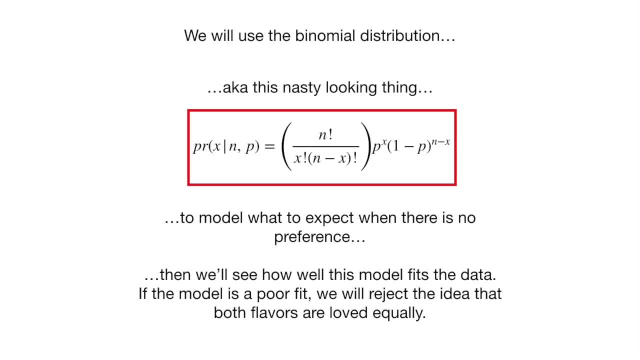 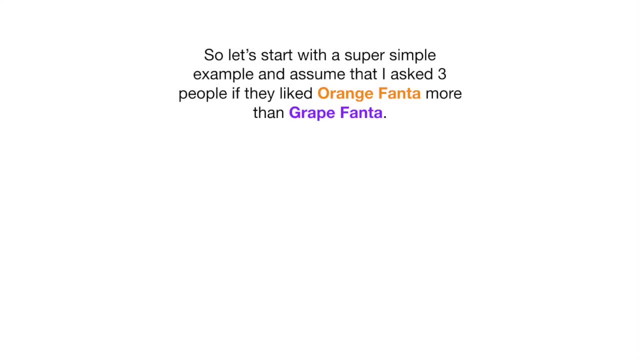 If the model is a poor fit, we will reject the idea that both flavors are loved equally. So let's start with a super simple example and assume that I asked three people if they liked orange Fanta more than grape Fanta. The first person we asked said they preferred orange Fanta. 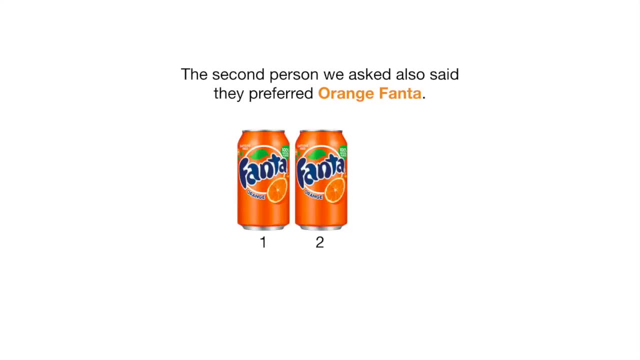 The second person we asked also said they preferred orange Fanta And the third person we asked said they preferred grape Fanta. If people really didn't prefer one flavor over the other, then we will assume that there is a 50% chance they will pick orange and a 50% chance they will pick grape. 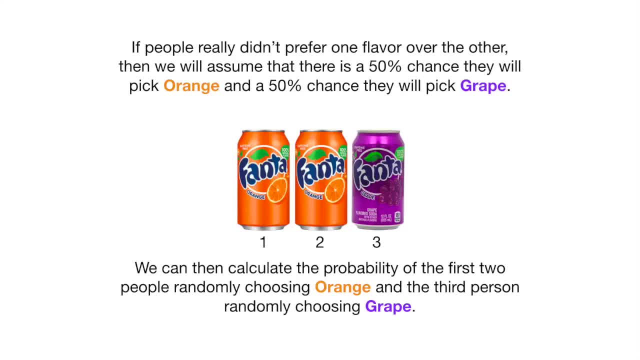 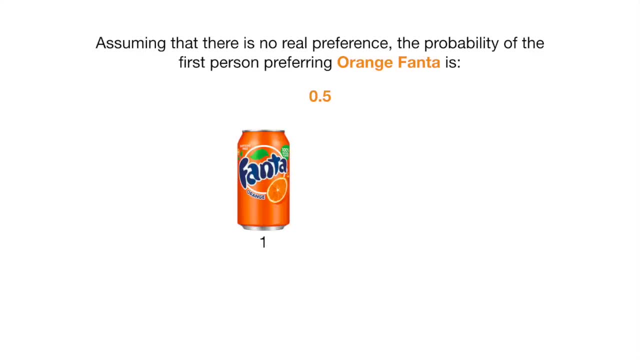 We can then calculate that. We can calculate the probability of the first two people randomly choosing orange and the third person randomly choosing grape, Assuming that there is no real preference. the probability of the first person preferring orange Fanta is 0.5. 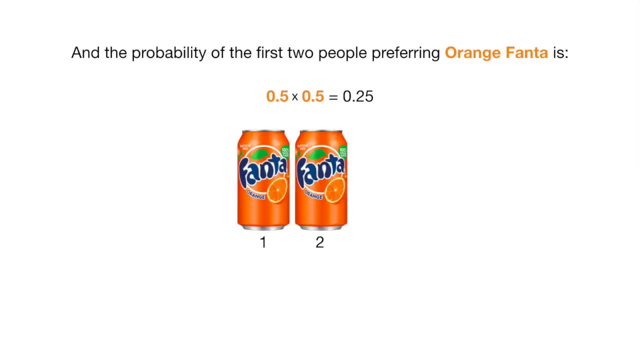 And the probability of the first two people preferring orange Fanta is 0.5 times 0.5, which equals 0.25.. And the probability of the first two people preferring orange Fanta and the third person preferring grape is 0.5 times 0.5 times 0.5, which equals 0.125. 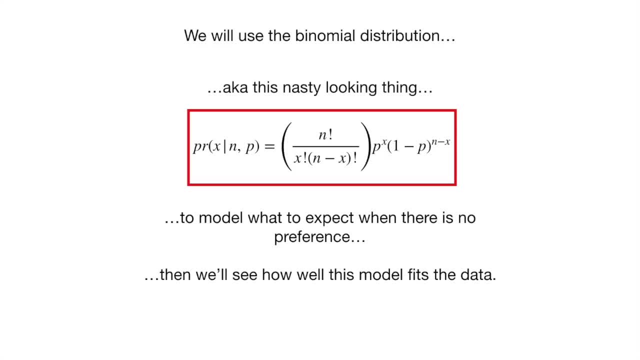 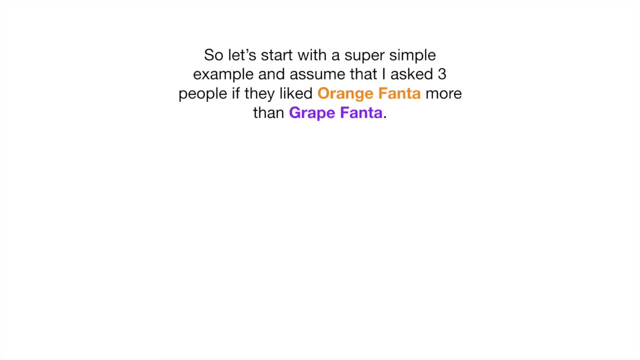 when there is no preference. Then we'll see how well this model fits the data. If the model is a poor fit, we will reject the idea that both flavors are loved equally. So let's start with a super simple example and assume that I asked three people if they. 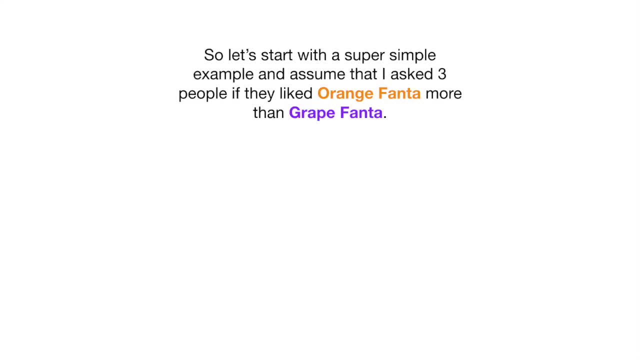 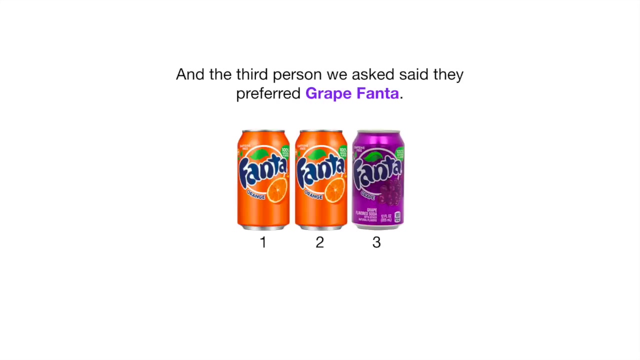 liked orange Fanta more than grape Fanta. To my하고 power Holzortimor. The first person we asked said they preferred orange Fanta. The second person we asked also said they preferred orange Fanta. And the third person we asked said they preferred grape Fanta. 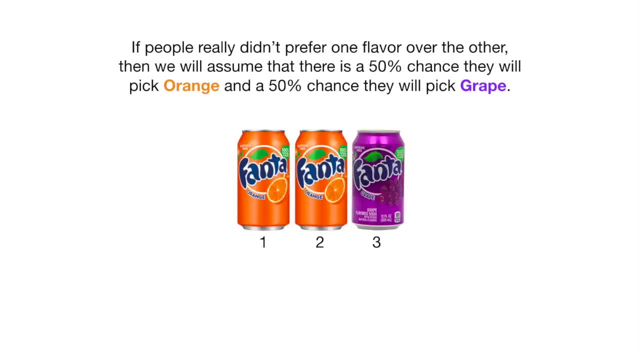 If people really didn't prefer one flavor over the other, then we will assume that there is a 50% chance they will pick orange and a 50% chance they will pick grape. We can then calculate the probability of the first two people randomly choosing orange. 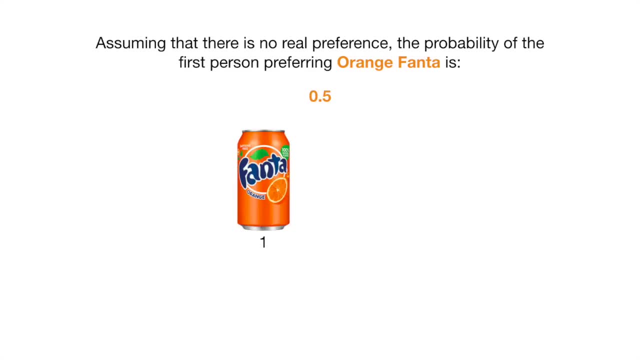 and the third person randomly choosing grape. Assuming that there is no real preference, the probability of the first person preferring orange Fanta is 0.5.. And the probability of the first two people preferring orange Fanta is 0.5 times 0.5,. 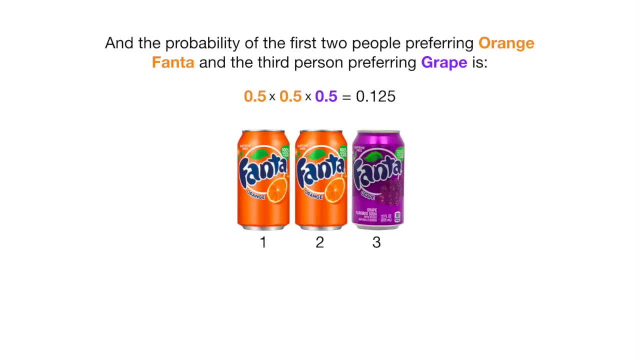 which equals 0.25.. And the probability of the first two people preferring orange, Fanta and the third person preferring grape is 0.5 times 0.5 times 0.5, which equals 0.125.. Note: 0.125 is the probability of the first two people saying they prefer orange and the. 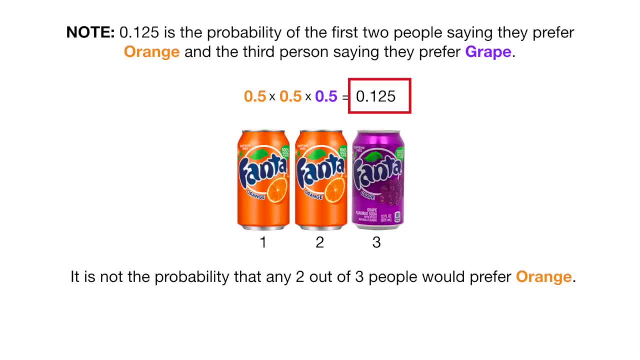 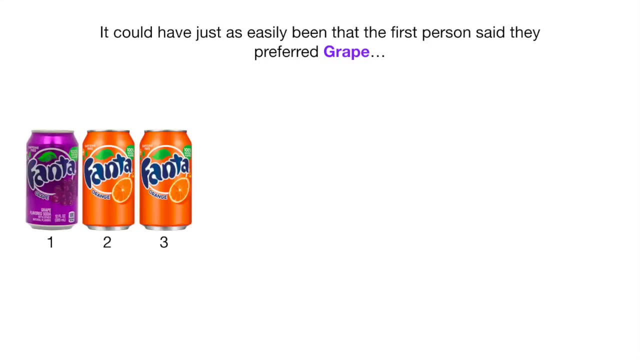 third person saying they prefer grape, the probability that any two out of three people would prefer orange. Let me explain: It could have just as easily been that the first person said they preferred grape. In this case the probability would still be 0.125, but 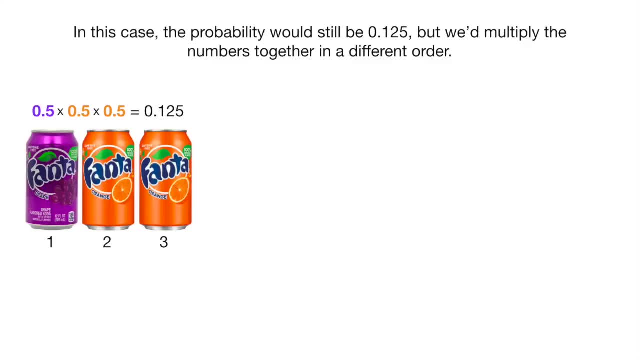 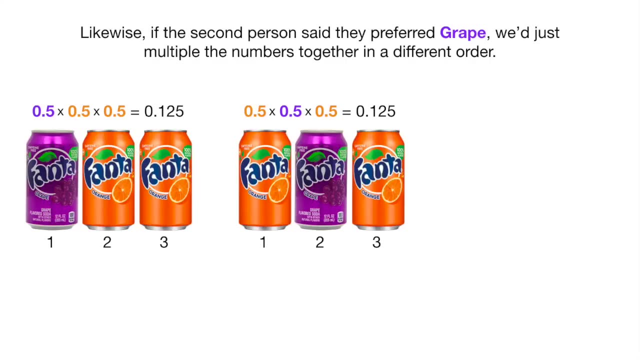 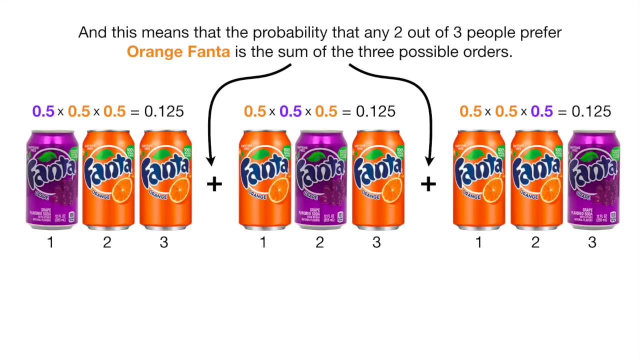 we'd multiply the numbers together in a different order. Likewise, if the second person said they preferred grape, we just multiply the numbers together in a different order. So all three of these combinations are equally likely and this means that the probability that any two out of three people prefer orange Fanta. 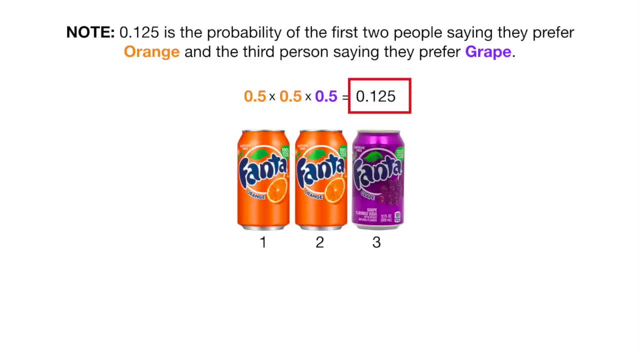 Note 0.125 is the probability of the first two people saying they prefer orange and the third person saying they prefer grape. It is not the probability that the first two people prefer orange and the third person prefer grape. It is the probability that any two out of three people would prefer orange. 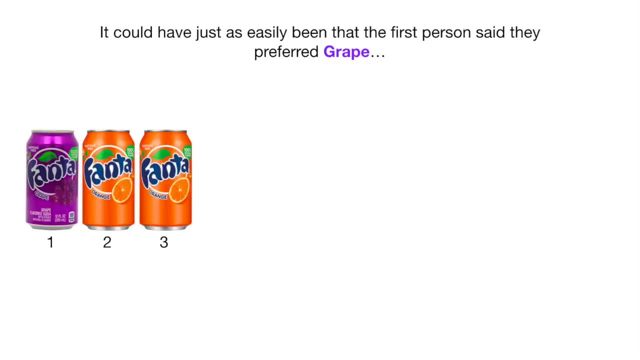 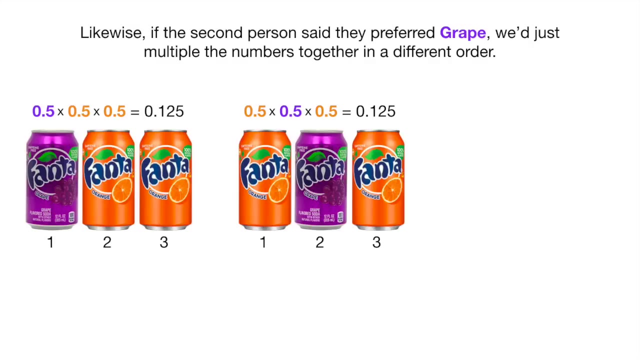 Let me explain. It could have just as easily been that the first person said they preferred grape. In this case, the probability would still be 0.125, but we'd multiply the numbers together in a different order. Likewise, if the second person said they preferred grape, we'd just multiply the numbers together. 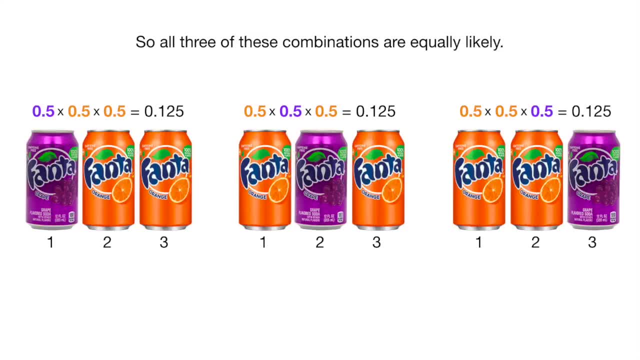 in a different order, So we'd add up 3 more people. Yes, So all 3 of these combinations are equally likely, And this means that the probability that any 2 out of 3 people prefer orange Fanta is the sum of the 3 possible orders. 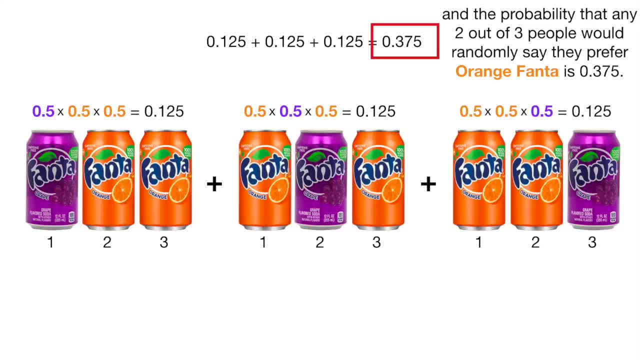 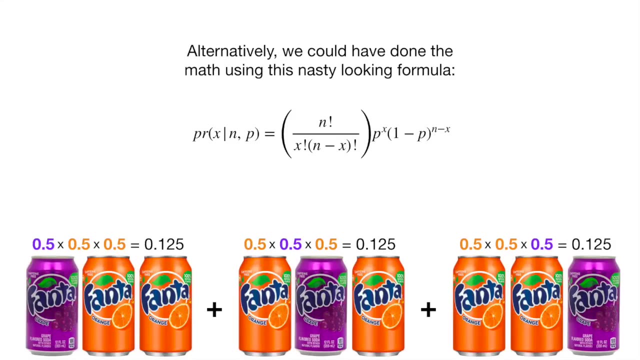 So we just add the three probabilities together And the probability that any 2 out of 3 people would randomly say they prefer orange Fanta is 0.375.. WTF. Alternatively, we could have done the math using this nasty-looking formula: 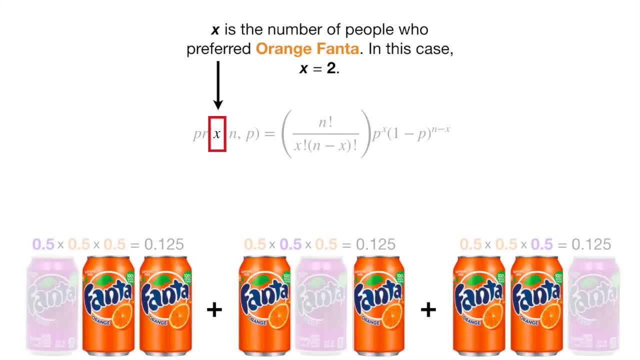 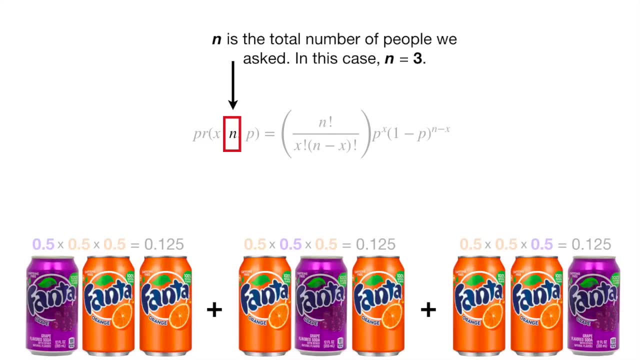 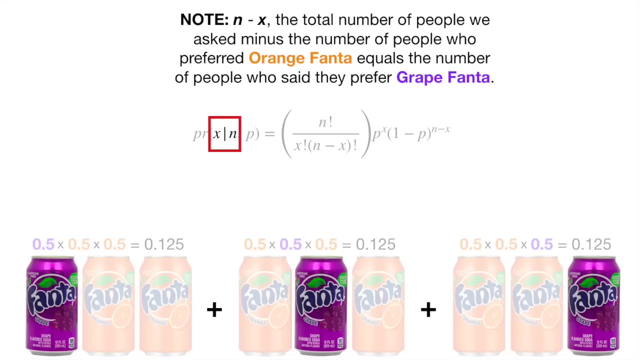 X is the number of people who preferred orange Fanta. In this case, X equals 2.. N is the total number of people we asked. In this case, N equals 3.. N minus X- the total number of people we asked, minus the number of people who. 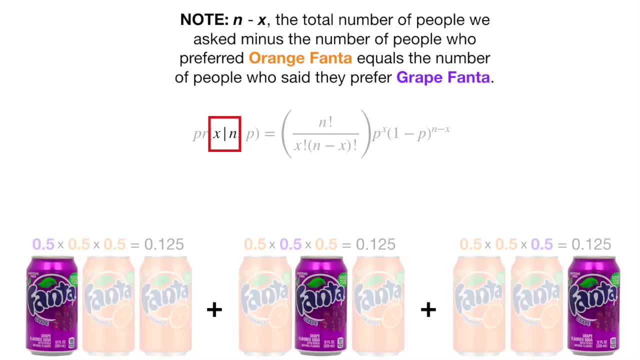 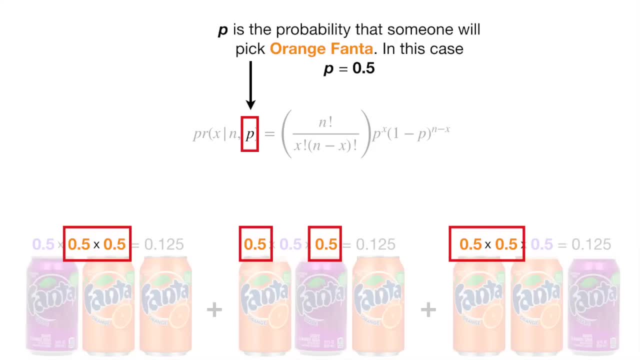 preferred orange Fanta equals the number of people who said they prefer grape Fanta. P is the probability that someone will pick orange Fanta. In this case, P equals 0.5.. the probability that someone might prefer grape Fanta is 1 minus P. 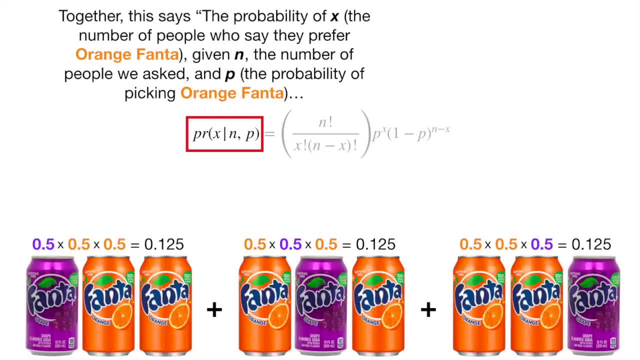 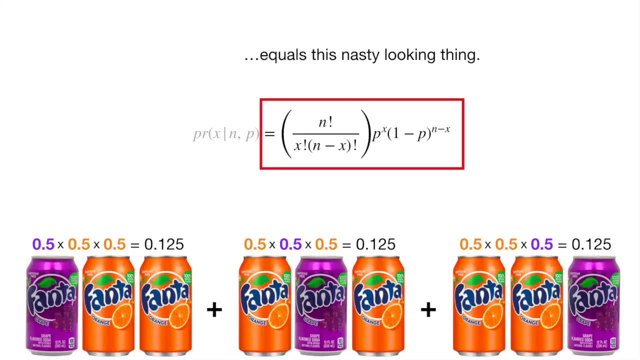 Together, this says the probability of X- the number of people who say they prefer orange Fanta. given N, the number of people we asked, and P- the probability of picking orange Fanta, equals this nasty-looking thing. Oooh, it's got factorials. 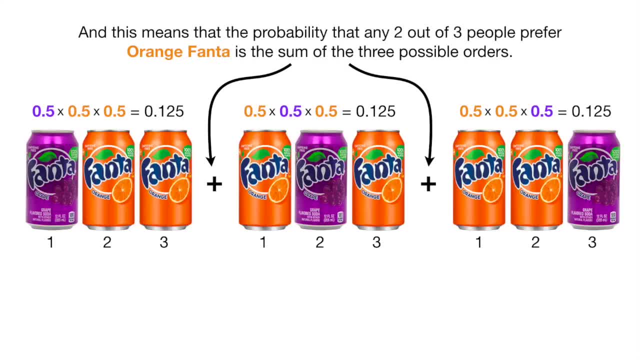 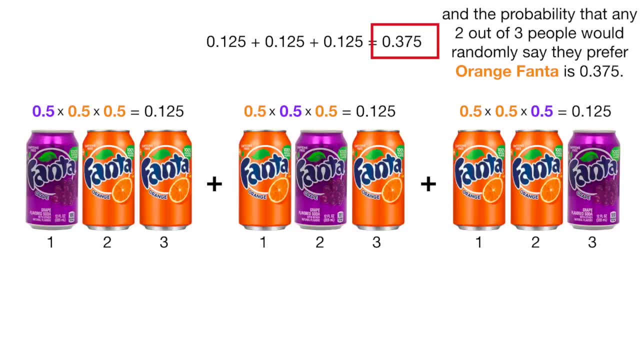 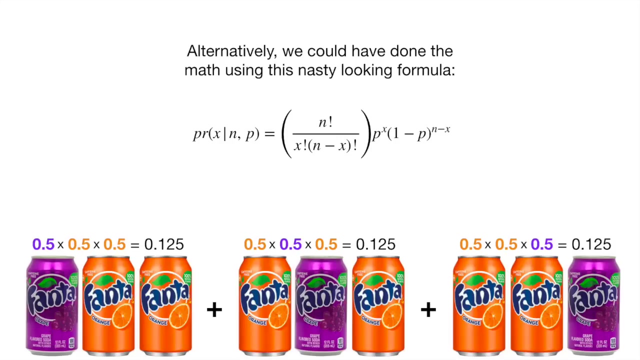 is the sum of the three possible orders. So we just add the three probabilities together and the probability that any two out of three people would randomly say they prefer orange Fanta is 0.375.. Alternatively, we could have done the math using this nasty-looking formula: 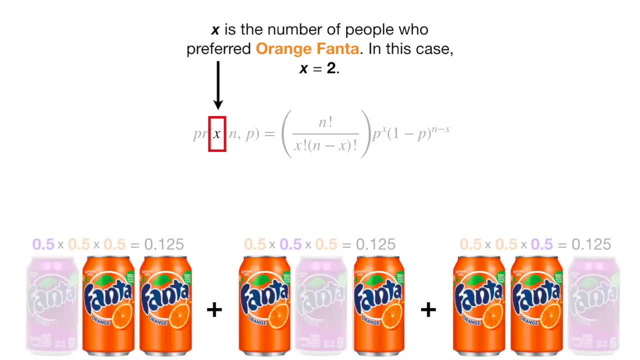 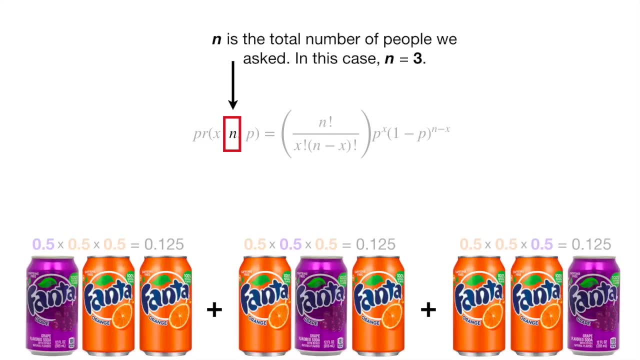 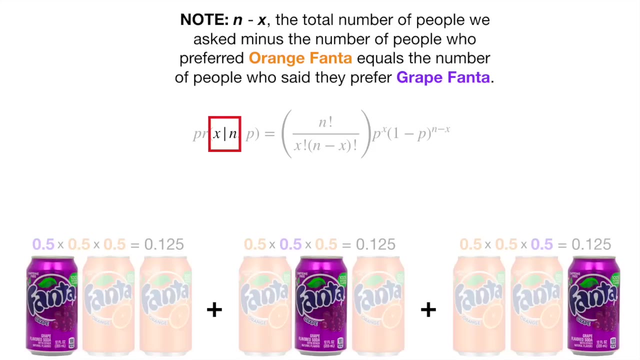 x is the number of people who preferred orange Fanta. In this case, x equals 2.. n is the total number of people we asked. In this case, n equals 3.. n minus x, the total number of people we asked. 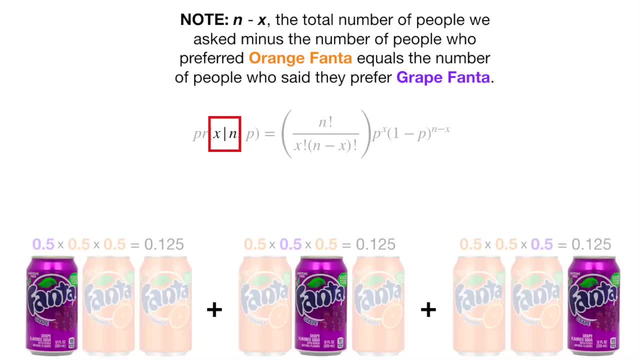 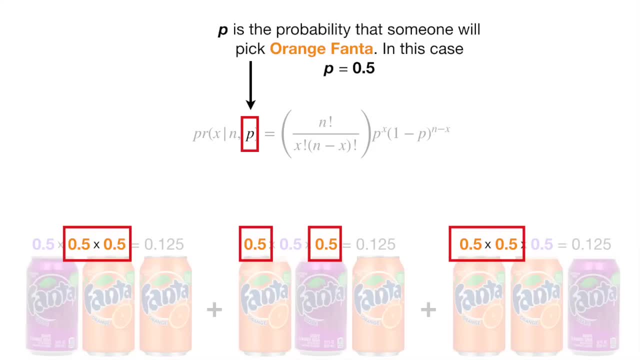 minus the number of people who preferred orange Fanta equals the number of people who said they prefer grape Fanta. p is the probability that someone will pick orange Fanta. In this case, p equals 0.5.. the probability that someone might prefer grape Fanta. 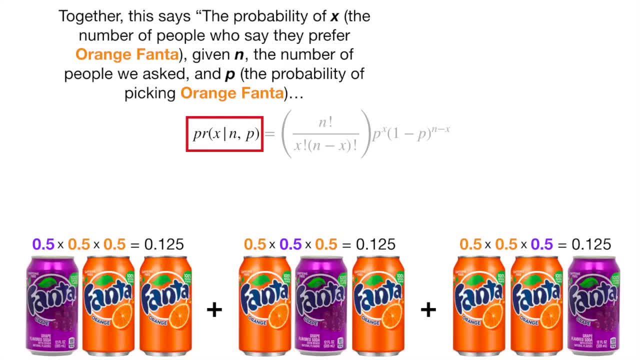 is 1 minus p. Together, this says the probability of x the number of people who say they prefer orange Fanta. given n the number of people we asked, and p the probability of picking orange Fanta, equals this nasty-looking thing. 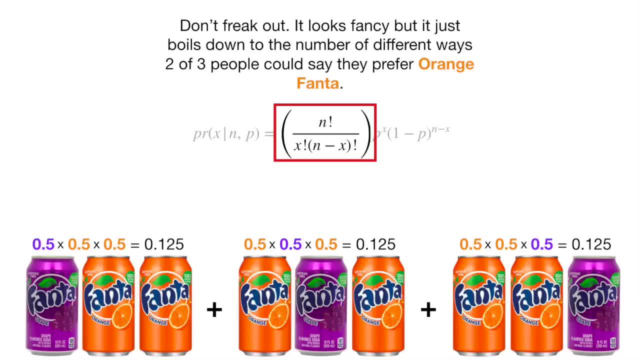 Oooh, it's got factorials. Don't freak out, It looks fancy, but it just boils down to the number of different ways. 2 of 3 people could say they prefer orange Fanta, When we did everything by hand. 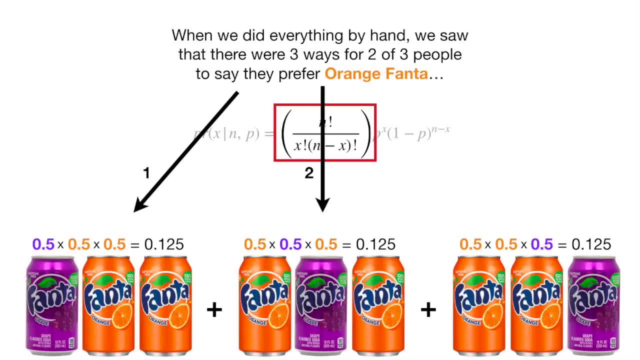 we saw that there were 3 ways for 2 of 3 people to say they prefer orange Fanta. And if we plug in n equals 3 and x equals 2, and then just do the math, we get 3.. We get 3.. 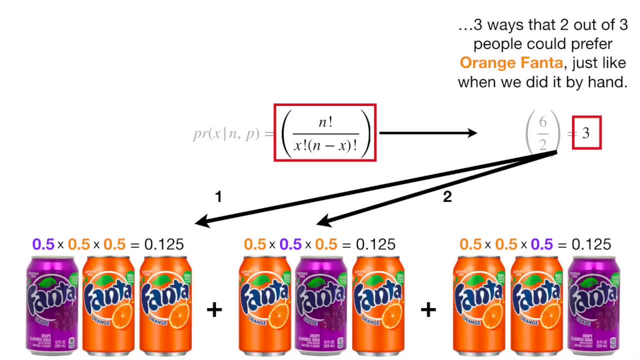 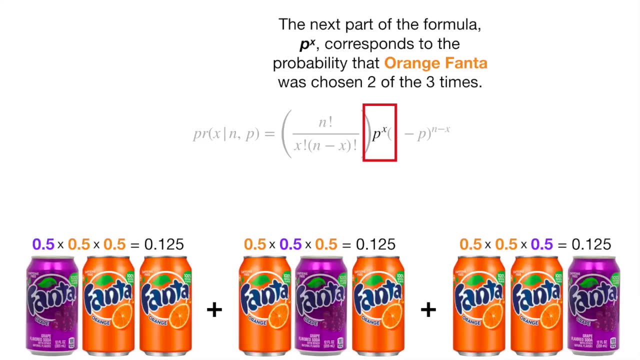 3 ways that 2 out of 3 people could prefer orange Fanta, just like when we did it by hand. So this fancy thing is really no big deal. The next part of the formula p to the x corresponds to the probability that orange Fanta was chosen 2 of the 3 times. 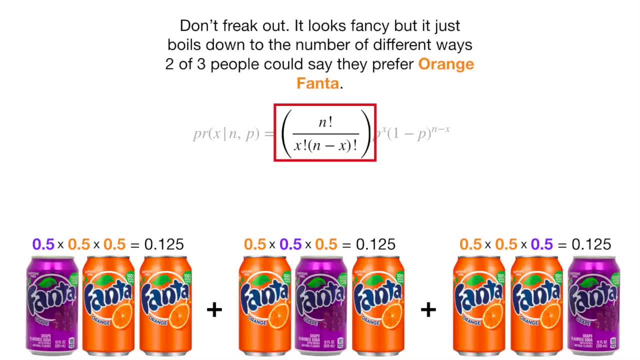 Don't freak out. It looks fancy but it just boils down to the number of different ways two of three people could say they prefer orange Fanta. When we did everything we could, we got the answer. When we did everything by hand, we saw that there were three ways for two of three people. 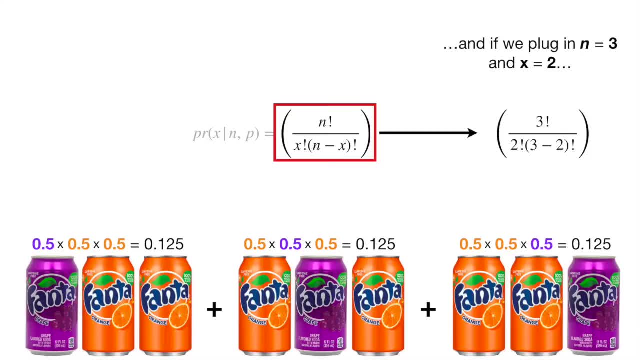 to say they prefer orange Fanta. And if we plug in N equals 3 and X equals 2, and then just do the math, we get 3.. Three ways that two out of three people could prefer orange Fanta, just like when we did. 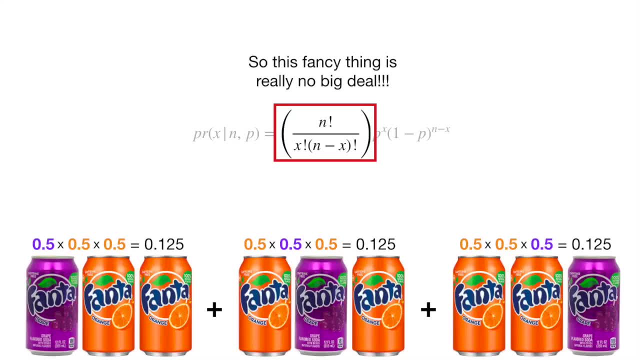 it by hand. So this fancy thing is really no big deal. The next part of the formula P to the X corresponds to the probability that orange Fanta was chosen two of the three times. In other words, P to the X just consolidates 0.5 times 0.5 into 0.5 squared. 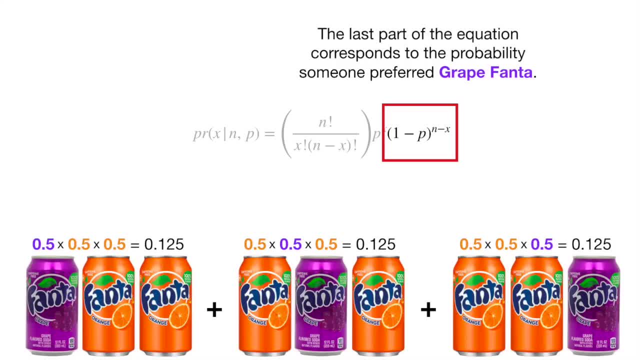 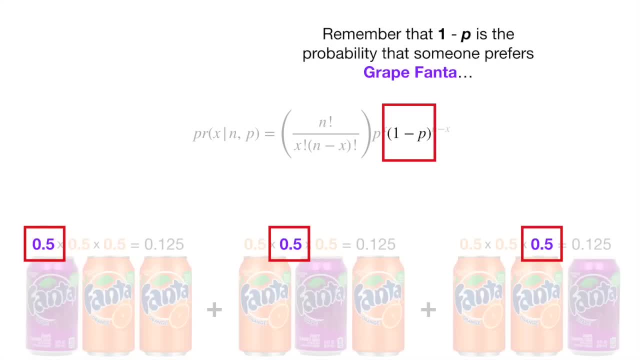 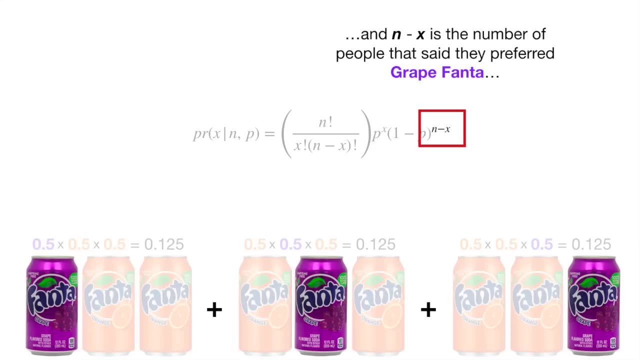 The last part of the equation is the formula. It corresponds to the probability that someone preferred grape Fanta. Remember that 1 minus P is the probability that someone prefers grape Fanta, And N minus X is the number of people that said they preferred grape Fanta. 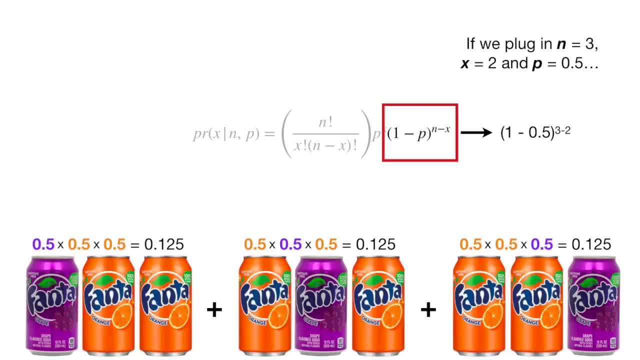 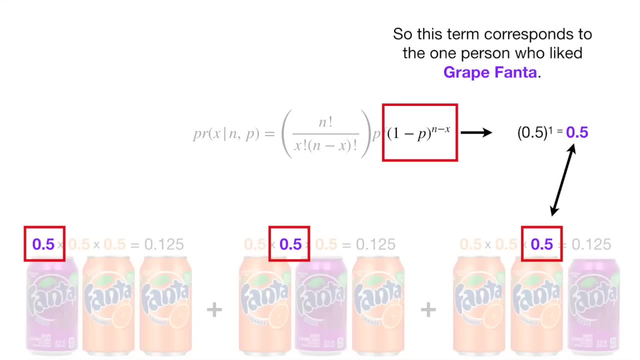 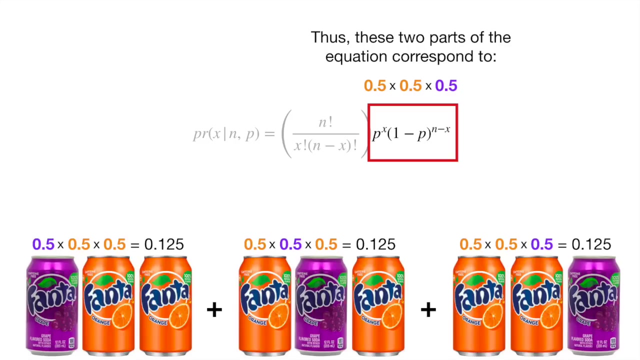 If we plug in N equals 3,, X equals 2, and P equals 0.5, and then do the math, we get 0.5. So this term corresponds to the one person who liked grape Fanta. Thus these two parts of the equation correspond to 0.5 times 0.5 times 0.5, and the nasty 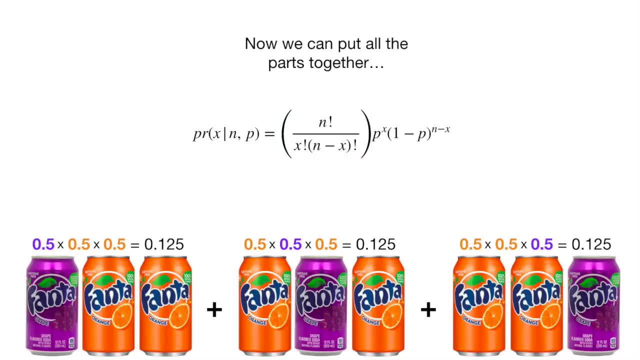 part just multiplies it by 3.. Now we can put all the parts together And plug in. X equals 2.. The number of people that preferred orange Fanta N equals 3. The number of people we asked, And P equals 0.5. 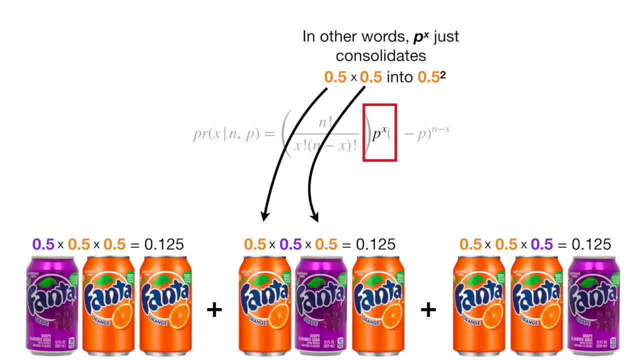 In other words, x just consolidates 0.5 times 0.5 into 0.5 squared. The last part of the equation corresponds to the probability that someone preferred grape Fanta. Remember that 1 minus p is the probability that someone. 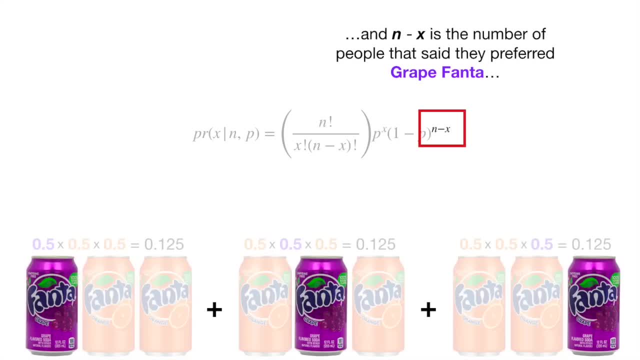 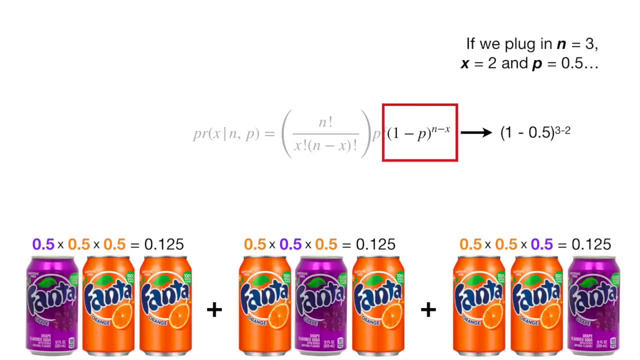 prefers grape Fanta And n minus x is the number of people that said they preferred grape Fanta. If we plug in n equals 3,, x equals 2, and p equals 0.5, and then do the math, we get 0.5. 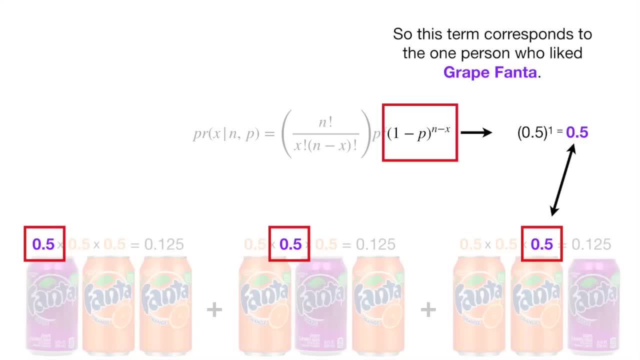 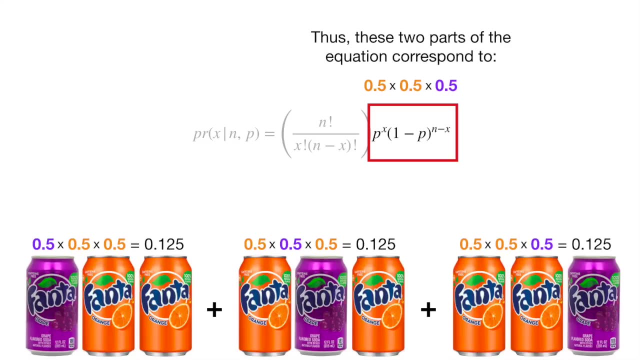 So this term corresponds to the one person who liked grape Fanta. Thus, these two parts of the equation correspond to 0.5 times 0.5 times 0.5.. 0.5 times 0.5 times 0.5.. 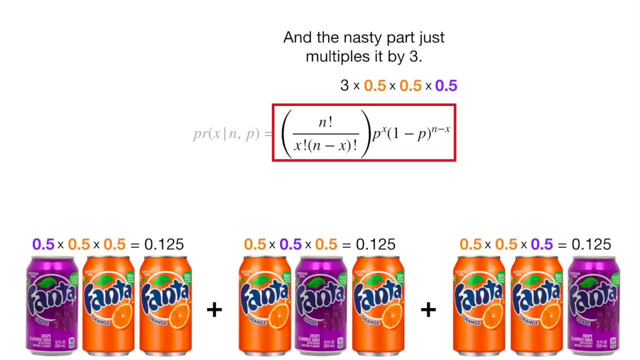 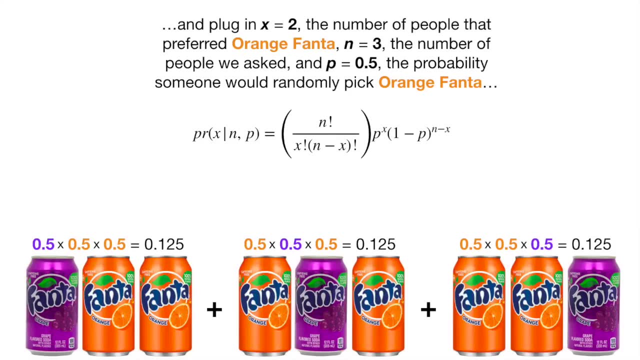 And the nasty part, just multiplies it by 3.. Now we can put all the parts together And plug in: x equals 2, the number of people that preferred orange Fanta n equals 3, the number of people we asked. 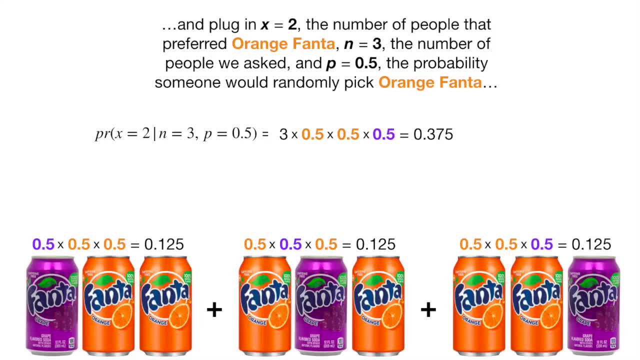 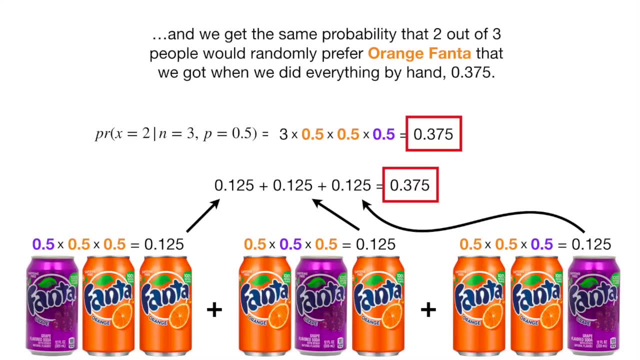 and p equals 0.5, the probability someone would randomly pick orange Fanta And we get the same probability that two of three people would randomly prefer orange Fanta that we got when we did everything by hand- 0.375.. In other words, the binomial distribution tells us that the probability 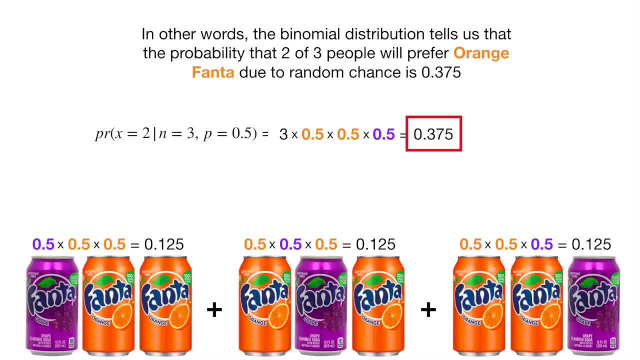 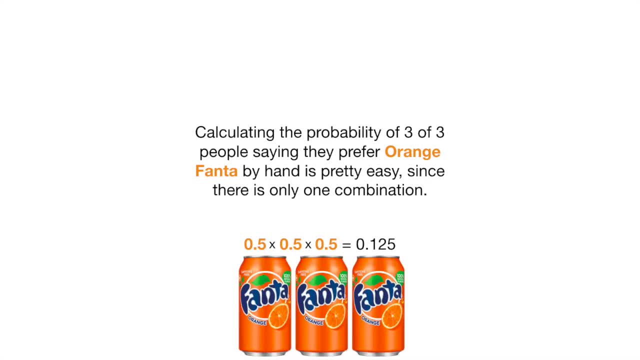 that two of three people will prefer orange Fanta due to random chance is 0.375.. BAM. So we can just as easily use the fancy formula by plugging in: x equals 3.. And then we just do the math: This term equals 1, since we are dividing 3 factorial by 3 factorial. 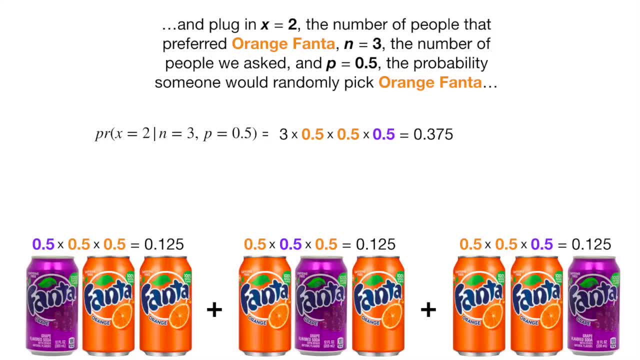 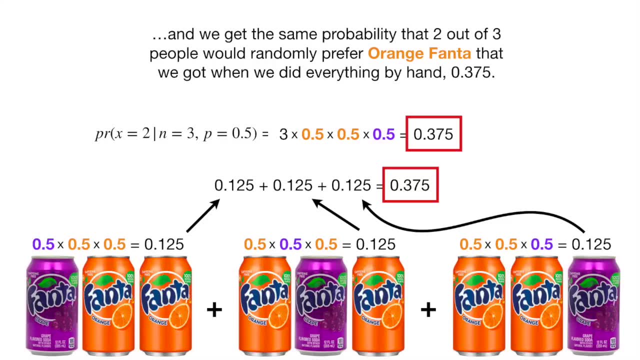 The probability someone would randomly pick orange Fanta And we get the same probability that 2 out of 3 people would randomly prefer orange Fanta that we got when we did everything by hand: 0.375.. In other words, the binomial distribution tells us that the probability someone chose 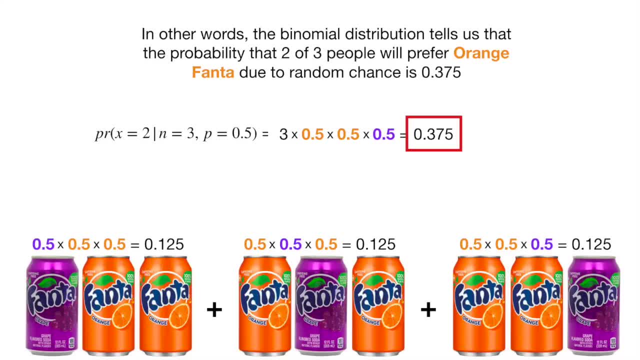 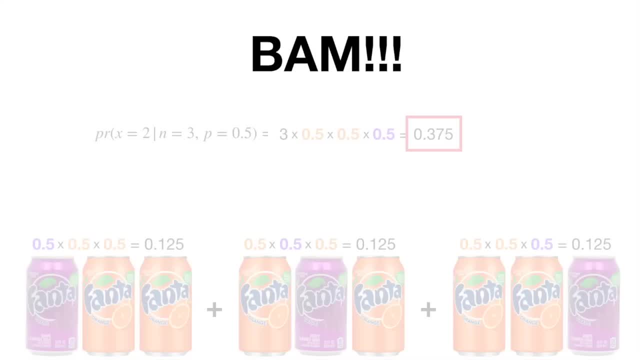 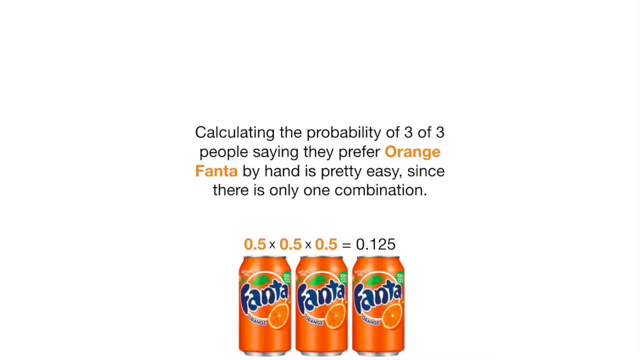 orange Fanta. would randomly choose orange Fanta. The probability that 2 of 3 people will prefer orange Fanta due to random chance is 0.375.. Bam, Calculating the probability of 3 of 3 people saying they prefer orange Fanta by hand is pretty easy. 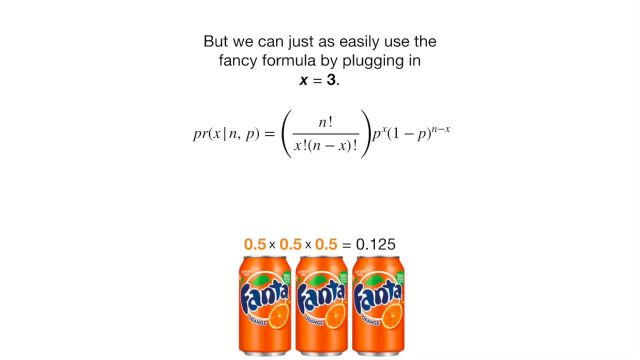 since there is only one combination. But we can just as easily use the fancy formula by plugging in: x equals 3, and then we just do the math: This term equals 1,, since we are dividing 3 factorial by 3 factorial. 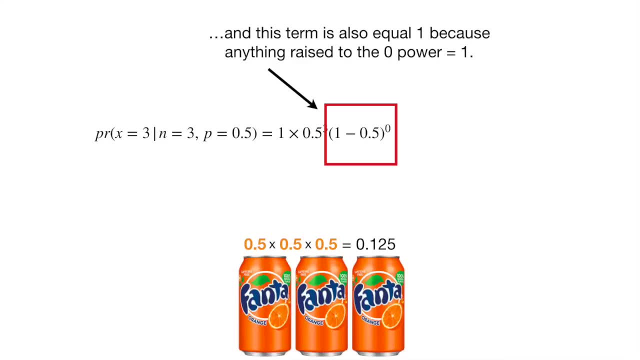 And this term is also equal 1, because anything raised to the 0 power equals 1.. And then we just keep doing the math And this means that the probability of 3 of 3 people randomly preferring orange Fanta is 0.375. 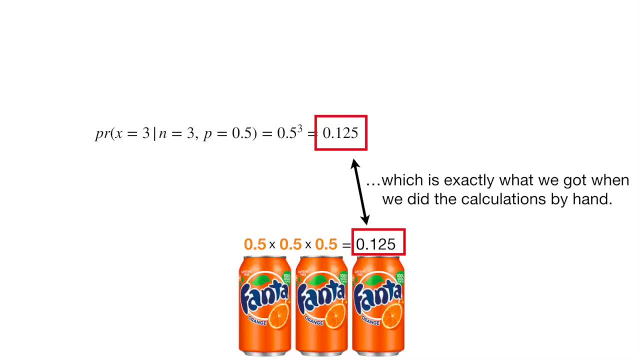 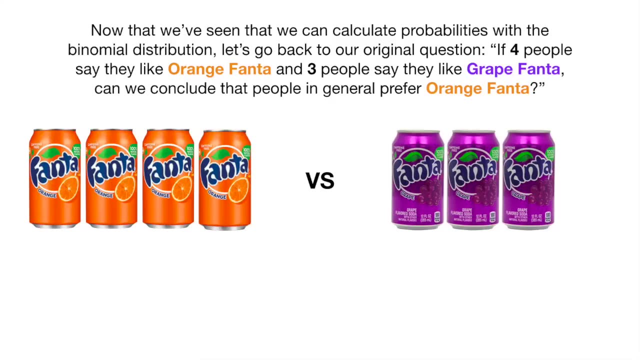 Which is exactly what we got when we did the calculations by hand. Now that we've seen that we can calculate probabilities with the binomial distribution, let's go back to our original question. If 4 people say they like orange Fanta and 3 people say they like grape Fanta, 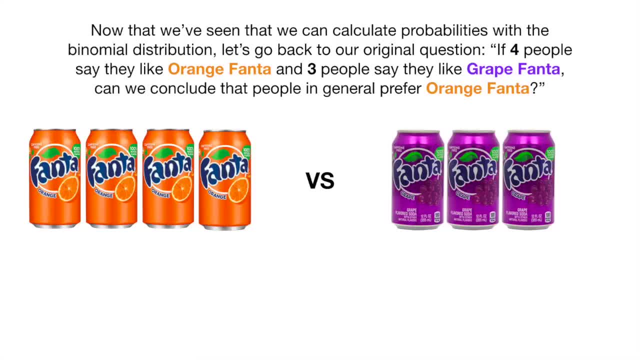 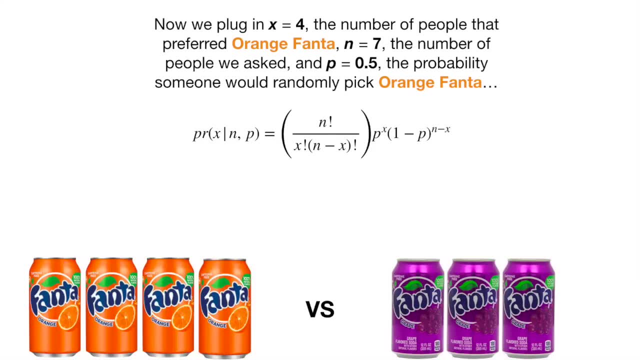 can we conclude that people in general prefer orange Fanta? Now we plug in: x equals 4, the number of people that preferred orange Fanta, n equals 7, the number of people we asked, and p equals 0.5,. 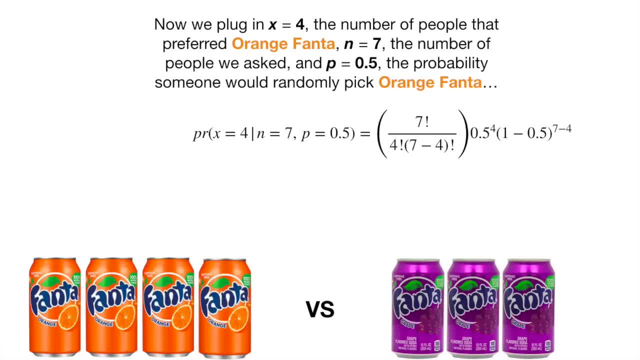 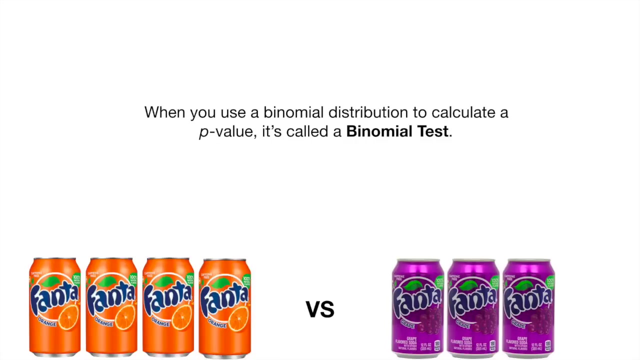 the probability someone would randomly pick orange Fanta And then just do the math And we get 0.273, the probability that 4 of 7 people would randomly prefer orange Fanta. Double bam When you use a binomial distribution to calculate a p-value. 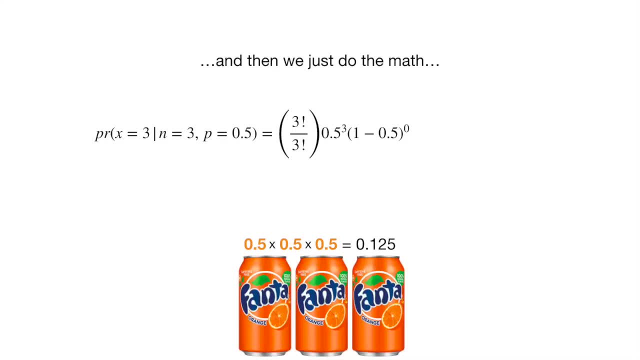 And this term is also equal 1,, because anything raised to the 0 power equals 1.. And this term is also equal 1,, because anything raised to the 0 power equals 1.. And this term is also equal 1,. 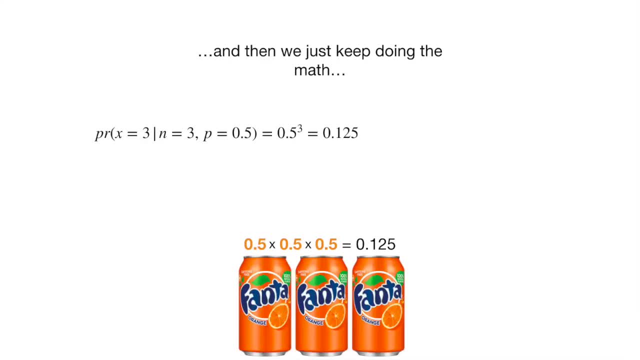 because anything raised to the 0 power equals 1.. And then we just keep doing the math And this means that the probability of three of three people randomly preferring orange Fanta is 0.125.. Which is exactly what we got when we did the calculations by hand. 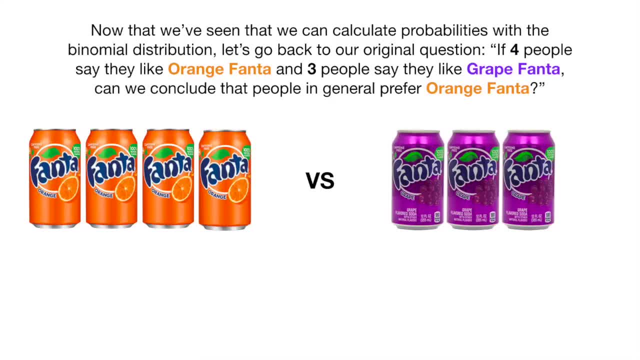 Now that we've seen that we can calculate probabilities with the binomial distribution, let's go back to our original question. If four people say they like orange Fanta and three people say they like grape Fanta, can we conclude that people in general prefer orange Fanta? 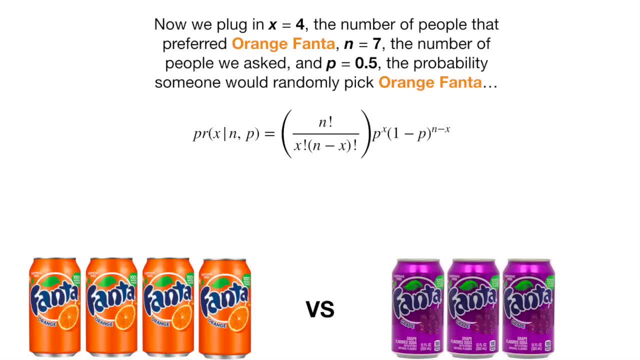 Now we plug in: x equals 4, the number of people that preferred orange Fanta n equals 7, the number of people we asked, and p equals 0.5,. what is the probability someone would randomly pick orange Fanta? 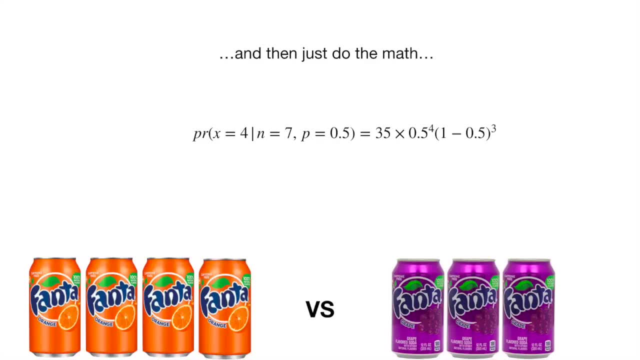 And then just do the math And we get 0.273, the probability that four of seven people would randomly prefer orange, Fanta, Double bam. When you use a binomial distribution to calculate a p-value, it's called a binomial test. 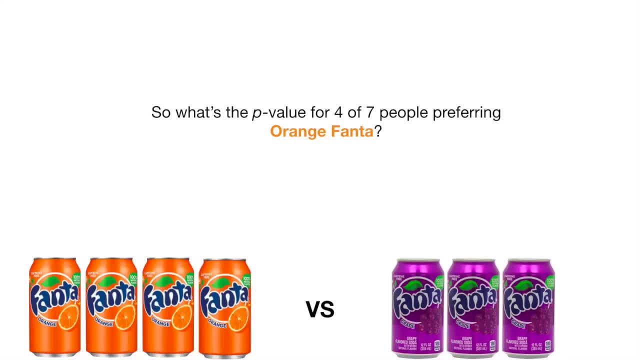 So what's the p-value for four out of seven people preferring orange Fanta? The p-value is the probability of the observed data plus the probabilities of all other possibilities that are equally likely or rarer. This means we need to calculate these probabilities. 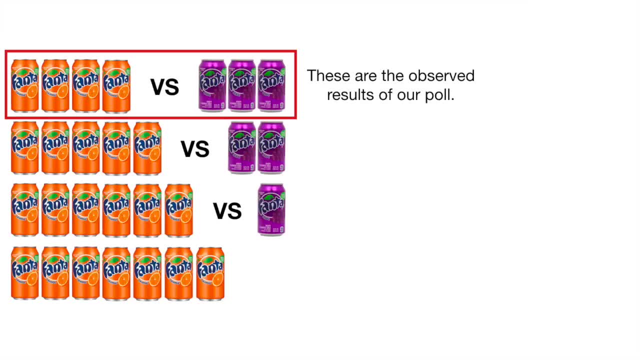 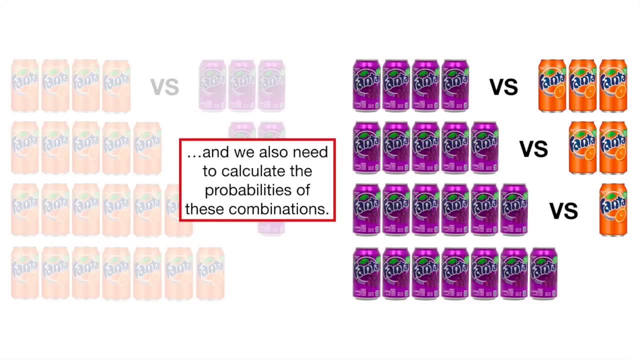 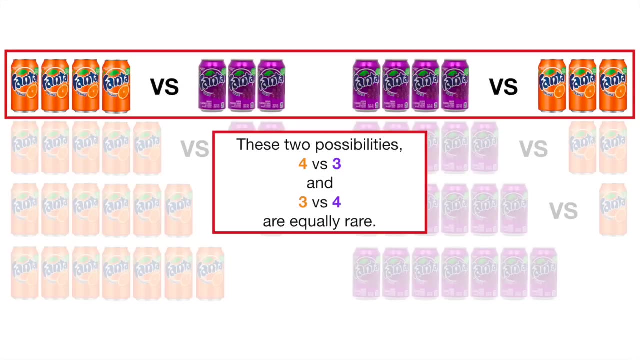 These are the observed results of our poll and these are rare possibilities And we also need to calculate the probabilities of these combinations. These two possibilities- 4 versus 3 and 3 versus 4, are equally rare. If you don't believe me, plug in the numbers and see. 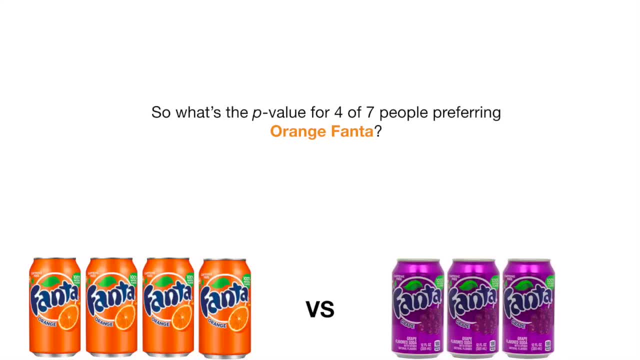 it's called a binomial test, So what's the p-value for 4 out of 7 people preferring orange Fanta? The p-value is the probability of the observed data- 4 of 7 people prefer orange Fanta- plus the probabilities of all other possibilities. 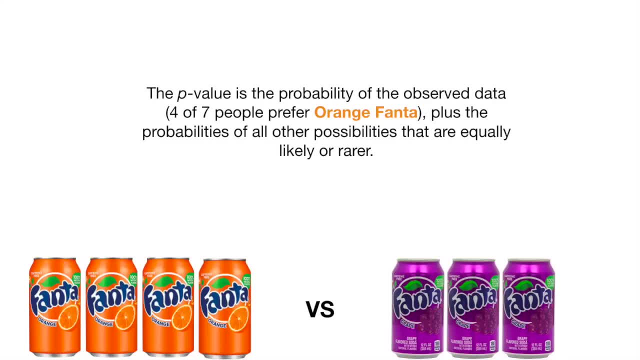 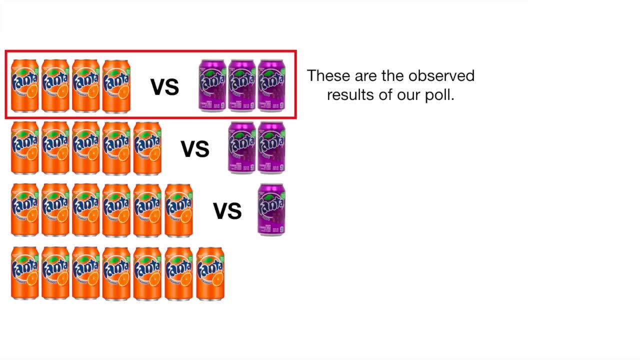 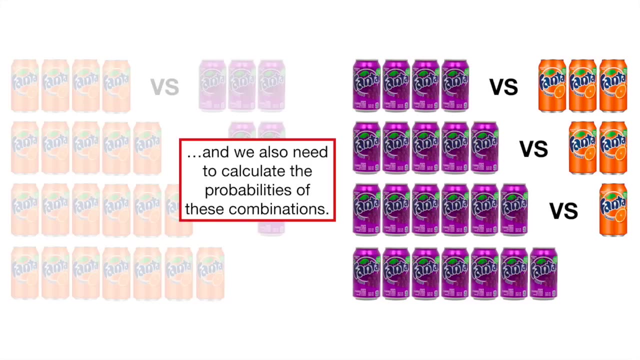 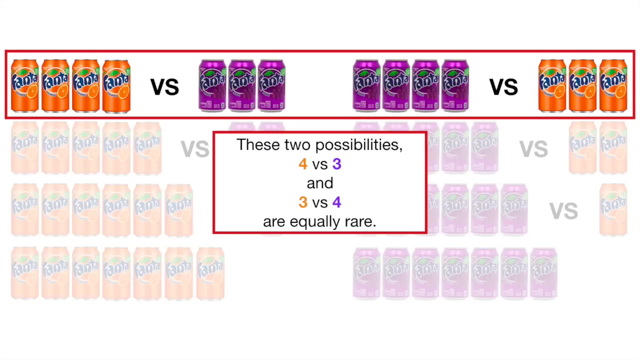 that are equally likely or rarer. This means we need to calculate these probabilities- These are the observed results of our poll and these are rare possibilities- And we also need to calculate the probabilities of these combinations, These two possibilities: 4 versus 3 and 3 versus 4,. 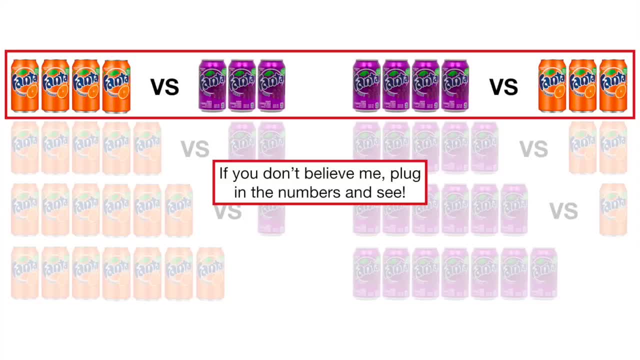 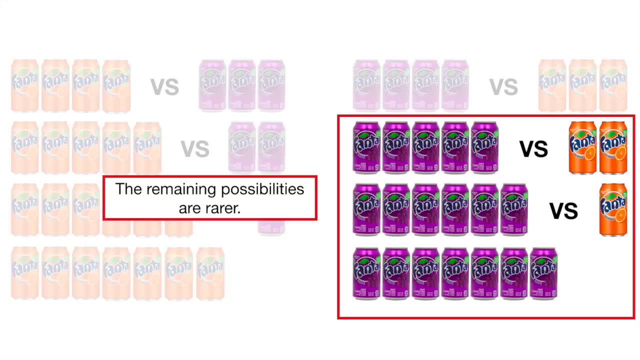 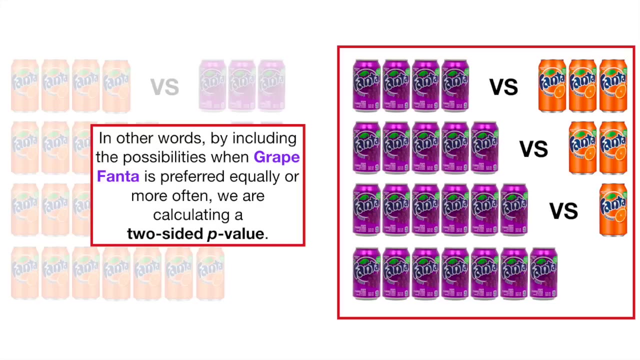 are equally rare. If you don't believe me, plug in the numbers and see. The remaining possibilities are rarer. In other words, by including possibilities when grape Fanta is preferred equally or more often, we are calculating a two-sided p-value. 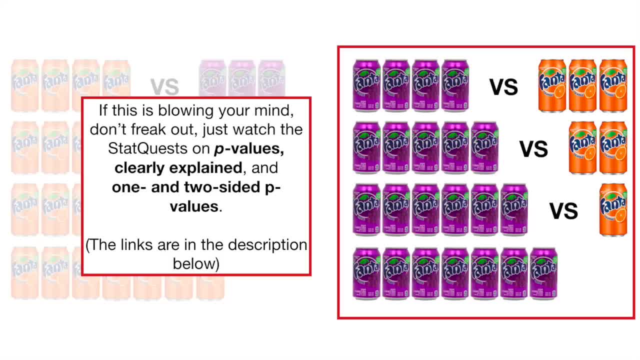 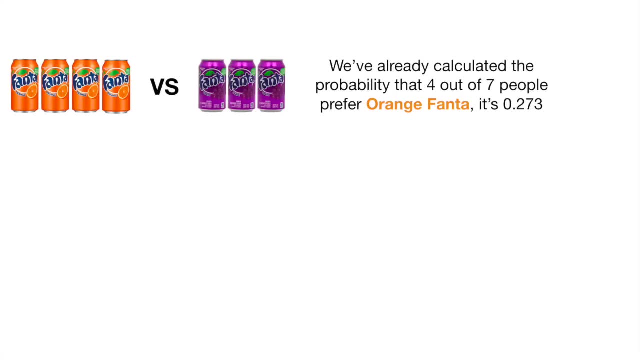 If this is blowing your mind, don't freak out. Just watch the StatQuest on p-values, which are already explained, and one- and two-sided p-values. The links are in the description below. We've already calculated the probability that 4 out of 7 people prefer orange Fanta. 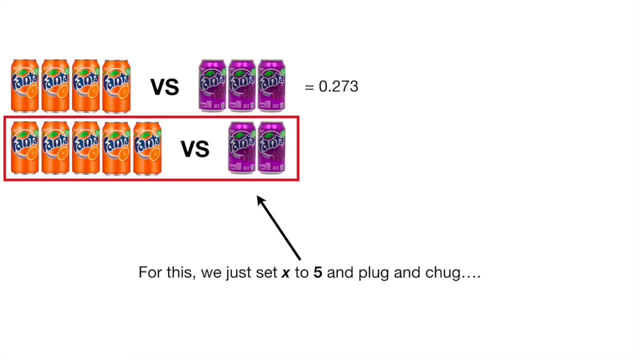 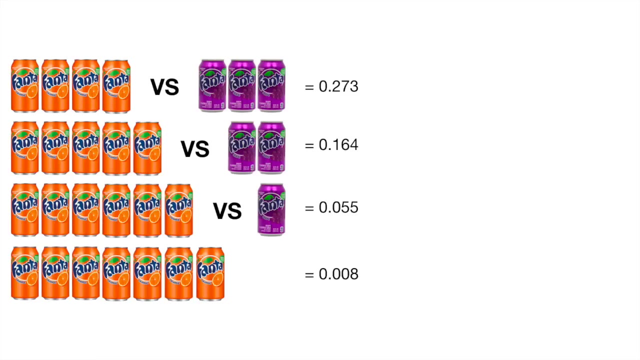 It's 0.273.. For this we just set x to 5 and plug and chug and we get 0.164.. Then we get 0.055, and then we get 0.008.. Adding the probabilities together gives us 0.5,. 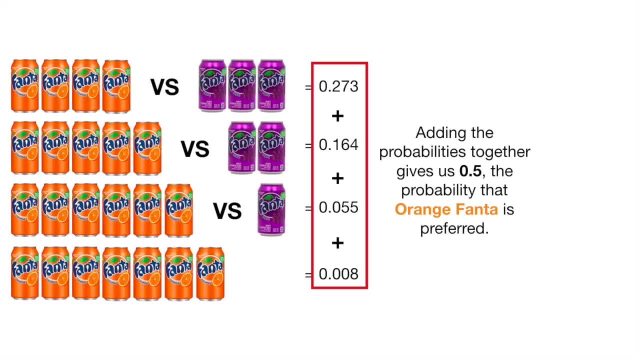 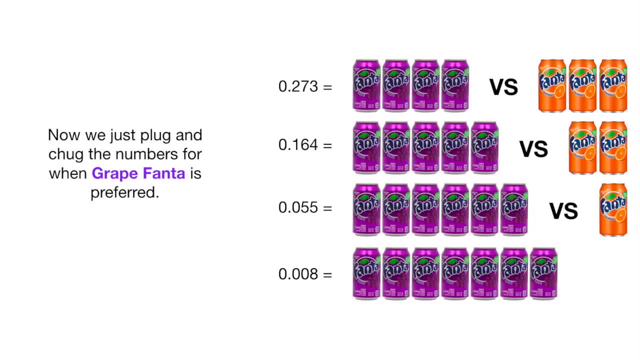 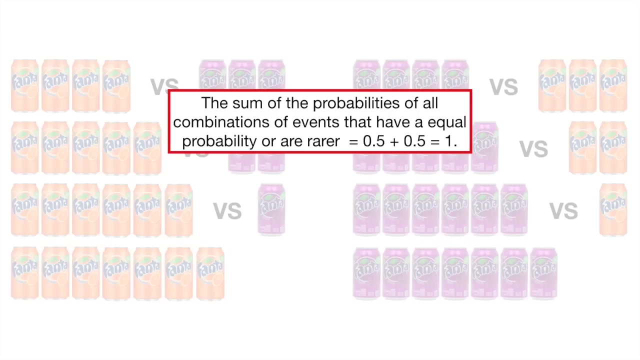 the probability that orange Fanta is preferred. Now we just plug and chug the numbers for when grape Fanta is preferred. Adding the probabilities together gives us 0.5, the probability that orange Fanta is not preferred, The sum of the probabilities of all combinations of events. 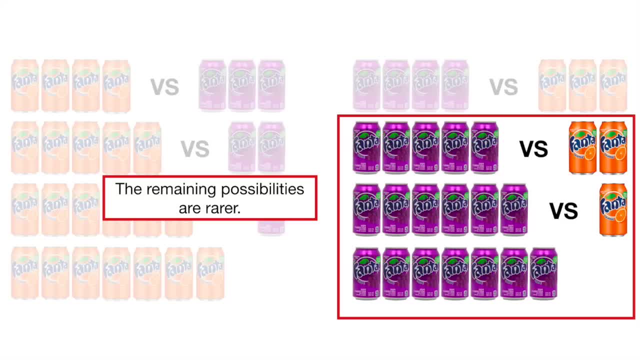 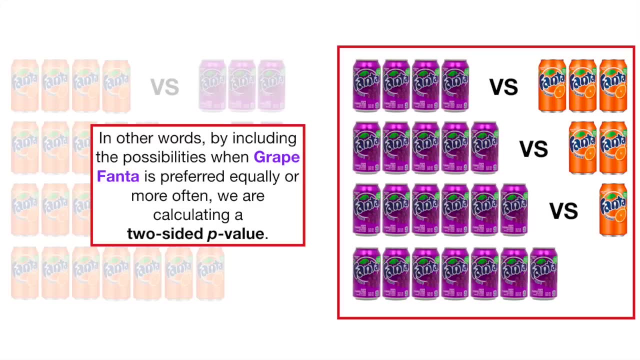 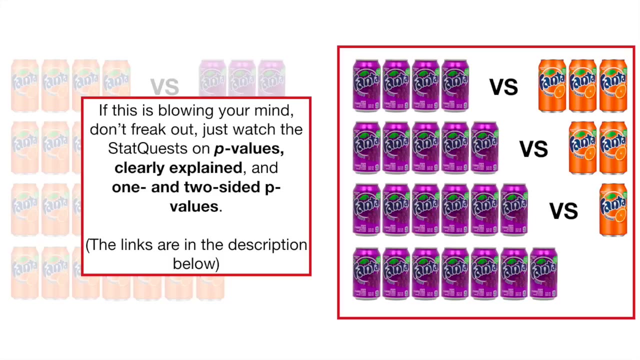 The remaining possibilities are rarer. In other words, by including possibilities when grape Fanta is preferred, equally or more often, we are calculating a two-sided p-value. If this is blowing your mind, don't freak out. Just watch the stat quest on p-values, clearly explained. 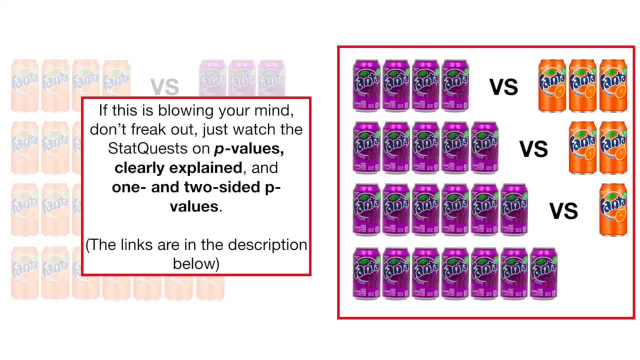 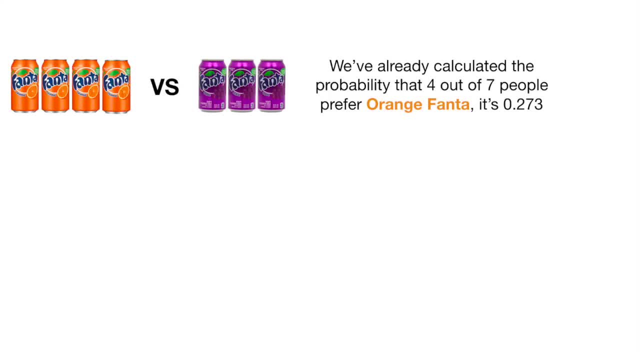 and one- and two-sided p-values. The links are in the description below. The links are in the description below. We've already calculated the probability that 4 out of 7 people prefer orange Fanta: It's 0.273.. 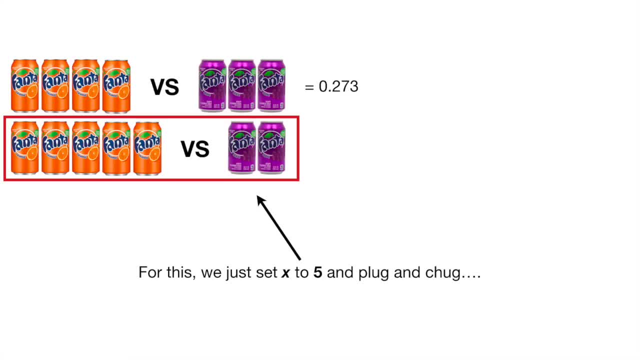 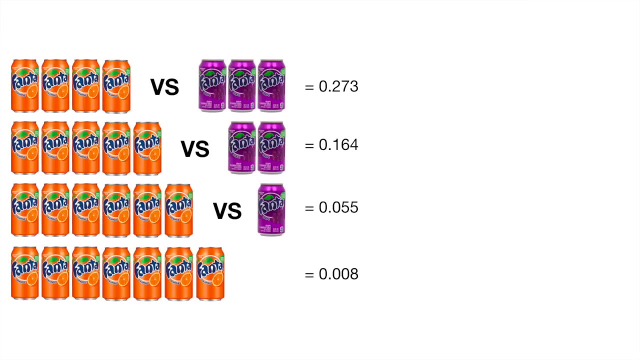 For this we just set x to 5 and plug and chug and we get 0.164.. Then we get 0.055, and then we get 0.008.. Adding the probabilities together gives us 0.5,. 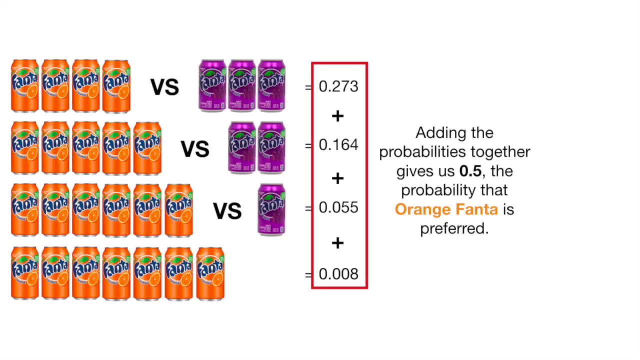 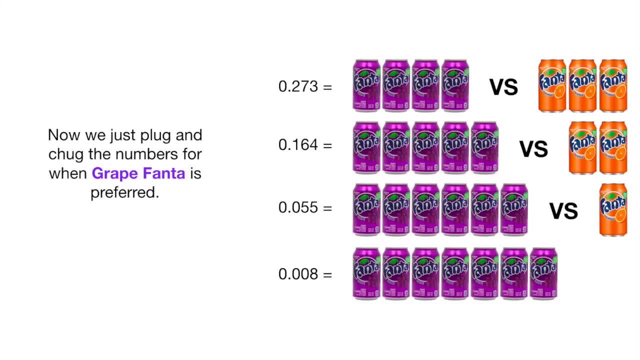 the probability that orange Fanta is preferred. Now we just plug and chug the numbers for when grape Fanta is preferred. Adding the probabilities together gives us 0.5, the probability that orange Fanta is not preferred, The sum of the probabilities of all combinations. 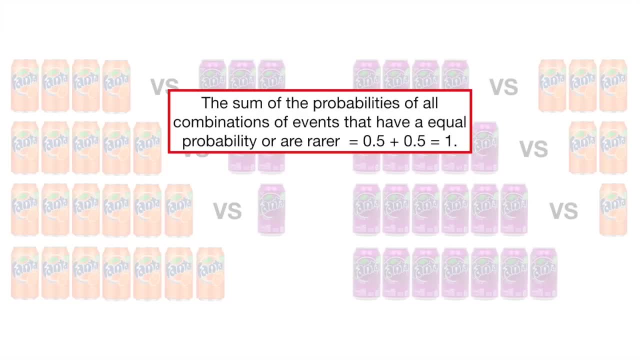 of events that have an equal probability or are rarer equals 0.5 plus 0.5, which equals 1.. Which means the p-value for 4 out of 7 people saying they prefer orange Fanta is 1., Which means that the model 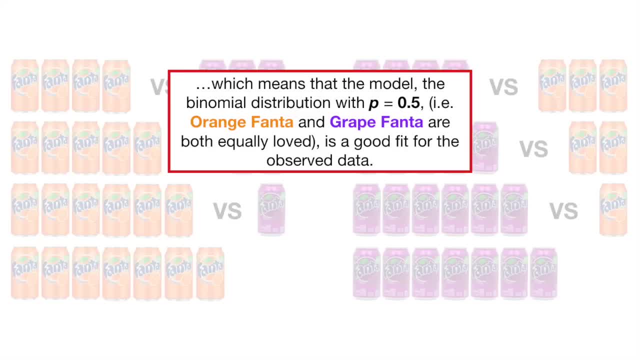 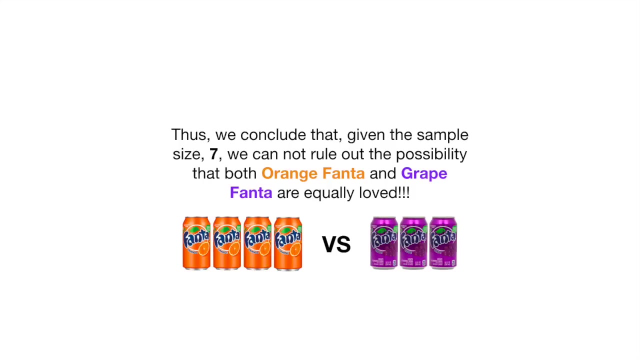 the binomial distribution with p equals 0.5,, ie orange Fanta and grape Fanta are both equally loved- is a good fit for the observed data. Thus we conclude that, given the sample size 7,, we cannot rule out the 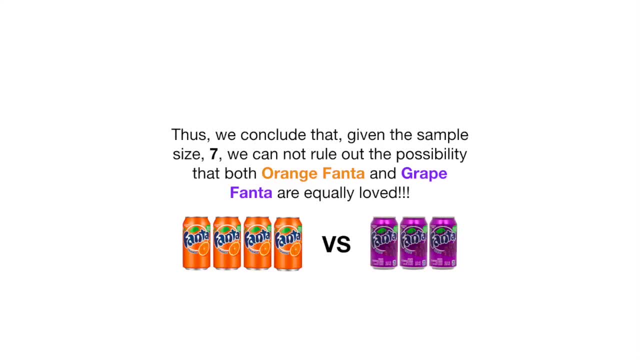 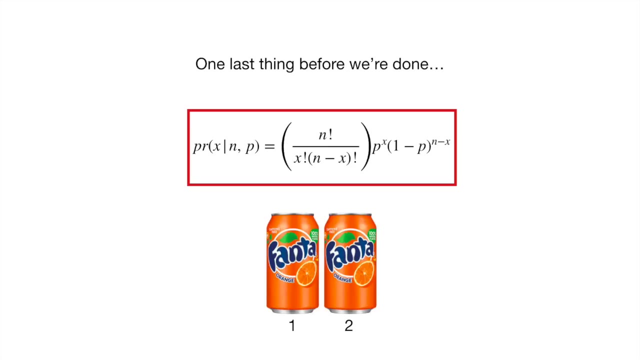 possibility that both orange Fanta and grape Fanta are equally loved. Think about that the next time you watch the World Series of Baseball Triple bam. One last thing before we're done. The binomial distribution only works when the probability that someone likes orange Fanta does not change if someone else.